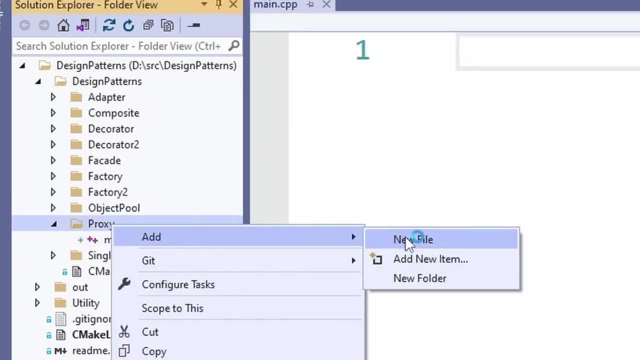 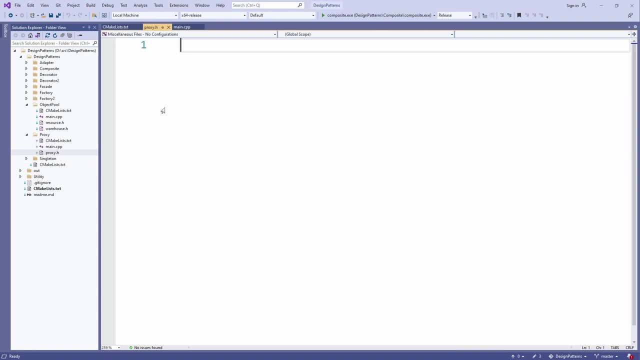 spot here in our repo link down below, and we're going to get this ready. Okay, and now, with all our CMake set up, we can go ahead and start showing an example. So I'm going to write all the example code here in this proxy folder. We need a subject to operate on. I'm going to use the idea of a store. 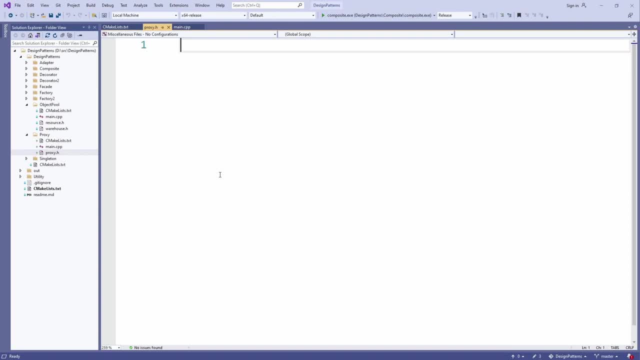 maybe an online store, and how they might or could tie some of their services together. Let's say, from the store you buy items that are for sale. So we're going to have class called item request. This is going to be an interface class. Now, what we want to do in this item request is essentially 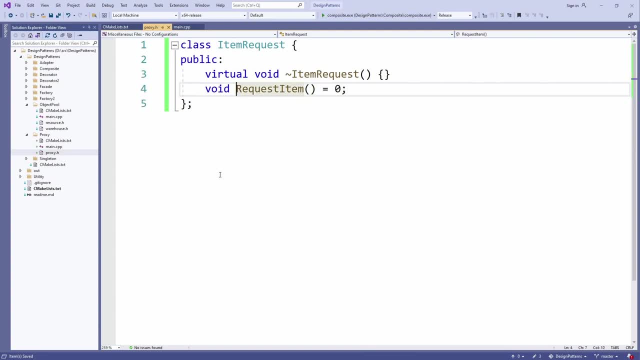 have a base request item. Let's make this all of it Now. we got to think about what happens when we request an item and what we might be doing here If we leave it pure virtual. that implementation is going to be left up to whoever implements this interface, But we could give it a root definition. 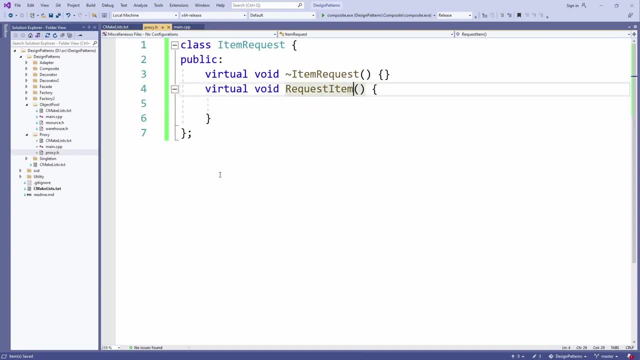 a base definition in case no one overrides it. So we're going to call it item skew. For simplicity sake, I'm just going to use integers and I'm going to use an integer called item skew. So essentially this would match with the available items. 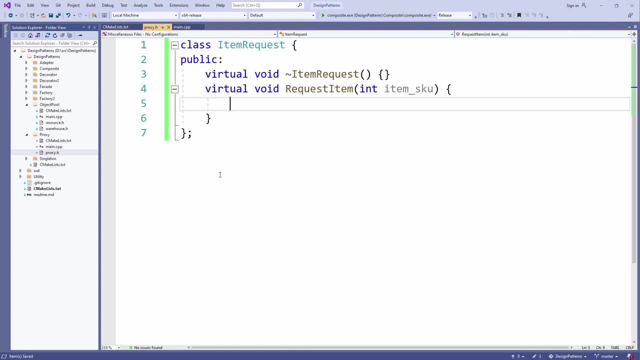 somewhere on a database. We're not going to build that database, but just to give you an idea of how it works. So you request an item and it returns void. That doesn't really work. We need to return something. So what we could do is we could also have a payment system, So that way it 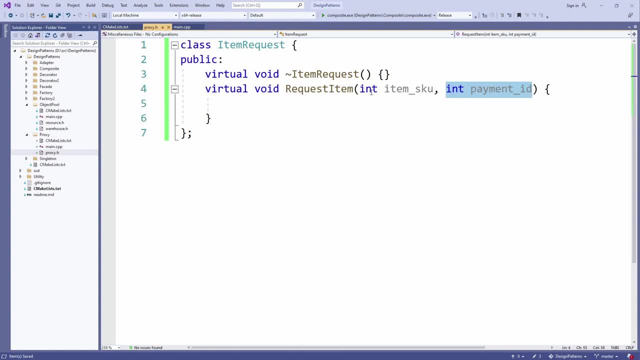 charges the payment system. Of course, this would probably be a more complicated struct, but we're just going to leave it as ID for now. We could even do it as a string, just for more details. But yeah, I think overall, if this were real, this would just be a struct that has some 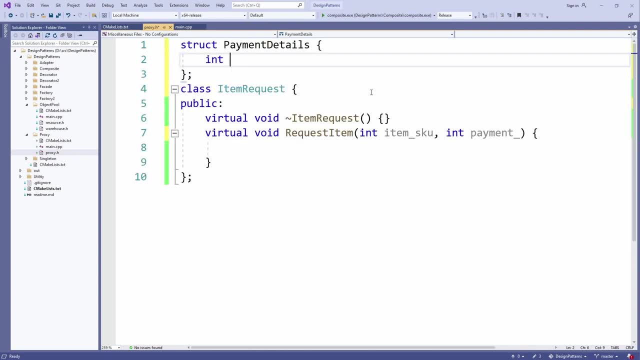 details. In fact, let's go ahead and build that. What would payment details have? We basically want to know whether it's like a bank or a card, credit card or something like that. Let's just go with. like you know, it's got to be some kind of digital pass in. There's no physical. 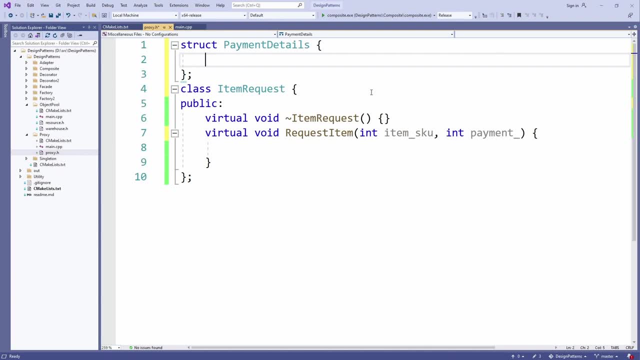 here in the code world. So no cash. So the payment details would have to be some basic thing like that. So, to avoid complications further, let's do some payment types and we're going to assume: well, we'll have credit card and we'll have bank. 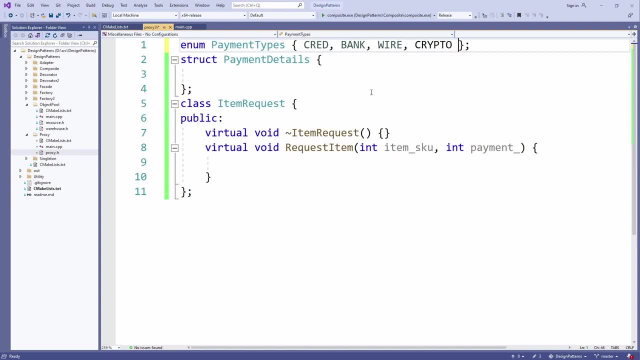 Or maybe we'll also have wire. Let's also put crypto in here, So let's say, we accept those types. Sounds good. Payment details is going to need a type and it's also going to need, I guess, something else. So we'd have to think about how we're putting this in here, I think. 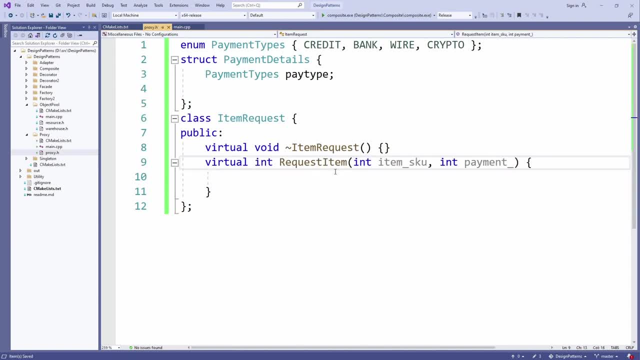 we're going to return just an integer or like the amount charged. So we could just have an interface, something like this: returns amount charged or zero if item is not found or payment could not be Okay. Well, I guess we could have different error codes. 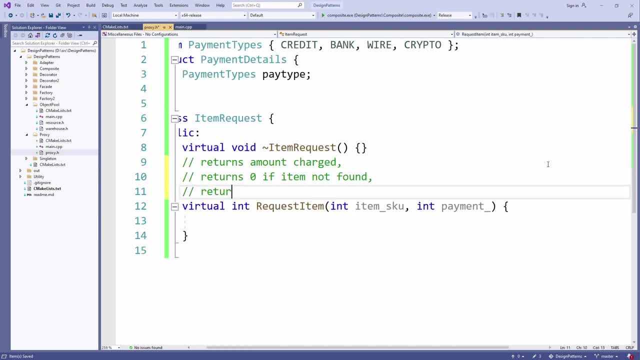 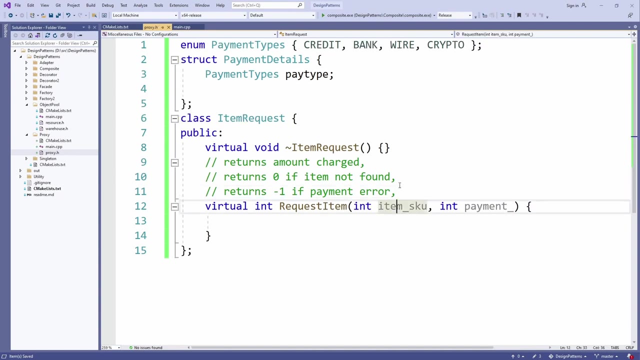 payable charged. returns zero if item is not found. Returns one if payment error: Well, not one, but negative one, And we could go on here. returns negative: two: Well, that's all we need for now. Payment error or item is not found Sounds good. 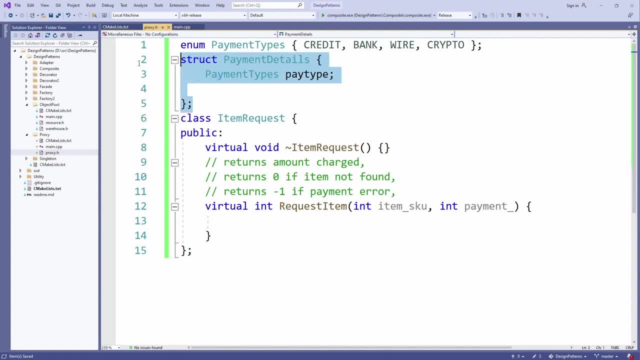 So we have this initial request item. Maybe we don't. Well, let's do this. If we pass this in by reference, we could edit their payment. So we don't necessarily to do that. so I think we're going to make it const and we're going to take it in as a copy. 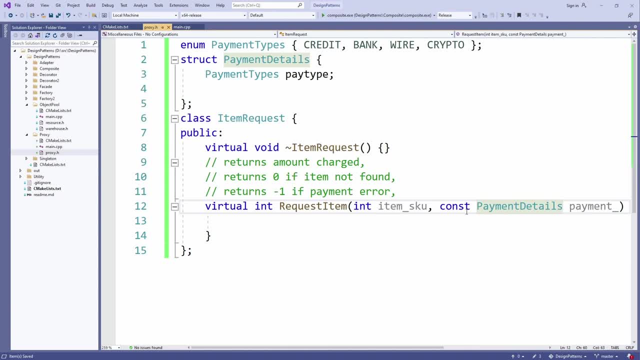 because we don't want any risk of any of these payment details getting changed. You could pass it in as a const reference and you think that might be fine, because, well, it's const and I have a reference to the real thing. but the problem here is in C++. it's a dangerous language. You can. 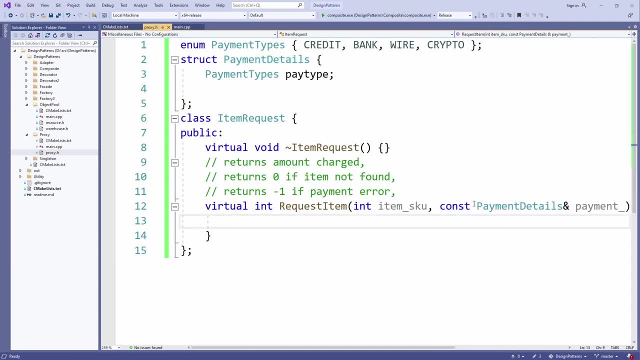 you can do a const cast and get rid of const and change the payment anyway. So for safety reasons we're just going to take in a copy so they can't change the real one coming in, and sure we'll make it const too. Items queue doesn't matter so much, but we'll make it const. It's a less security. 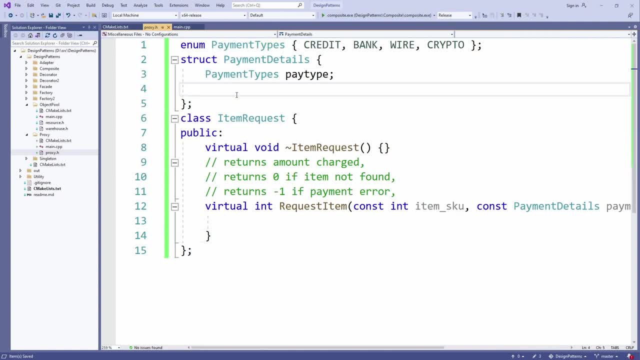 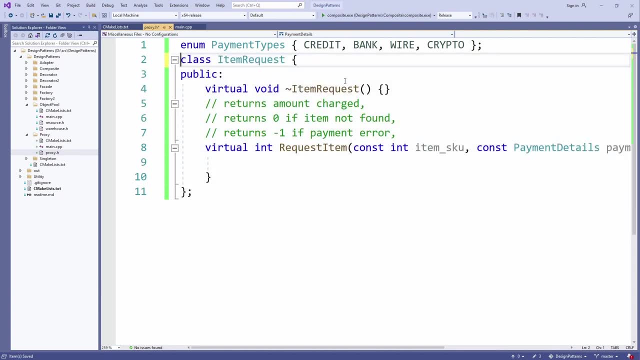 intensive asset. Maybe we only need pay type, but yeah, let's just go with pay type. We don't need these details. after all, Payment types is good enough, and in this code we're going to pseudo code up a few things but pretend this is. 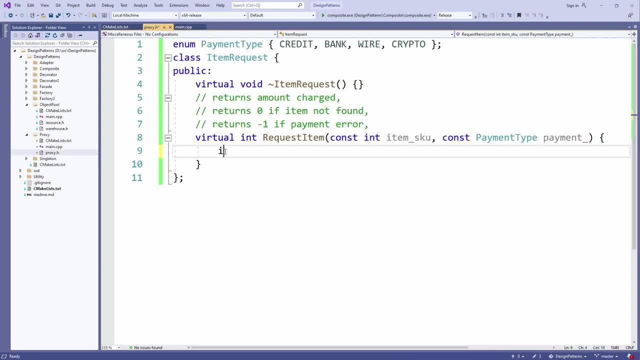 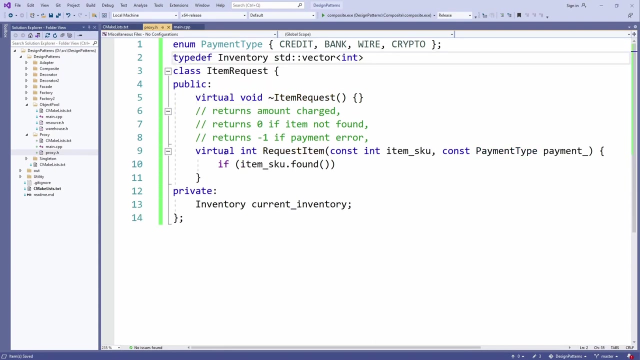 talking to some kind of database. So we go if- but you know before this- we might actually have to connect to something like a database, or maybe it would just be like that: Let's go with inventory and for this inventory let's type def inventory as a vector of ints. So now this is just a vector. 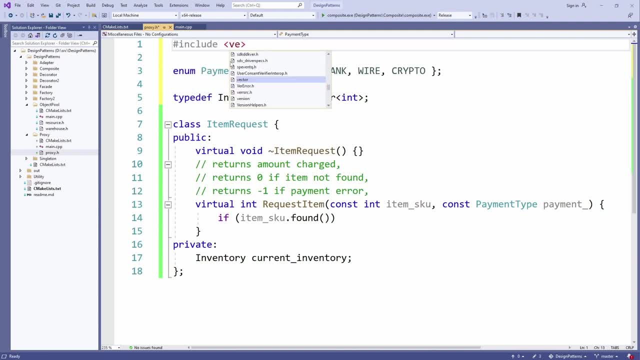 go ahead and include anything you need up here: Vector. So basically this would be more like a database link, but let's keep it simple here. So we go something like the current query: What is the function? I forget. So we can use standard find here. 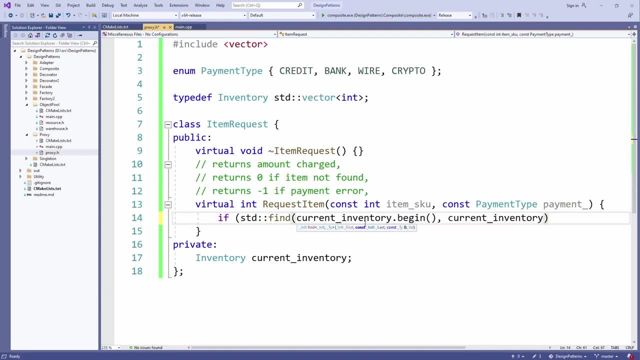 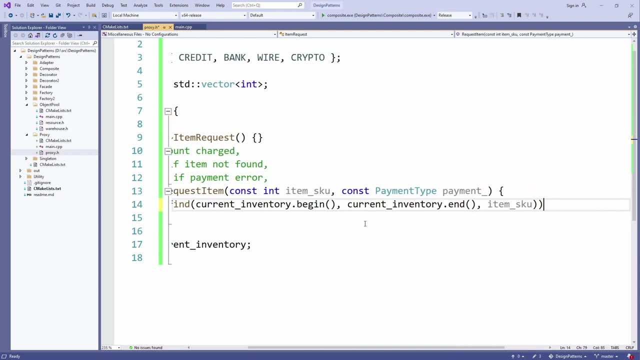 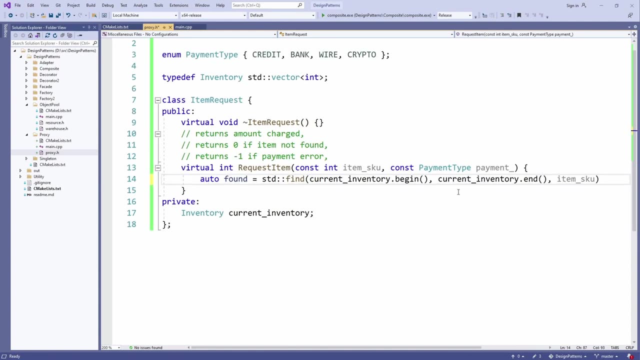 starting with the beginning of the inventory to the end of the event inventory and then what we're looking for, which is the item skewed. so if this returns- not the end, so it'd probably be better to do this on its own line at first, a moment when you're too zoomed in, just trying to make sure it's invisible, all right. so this 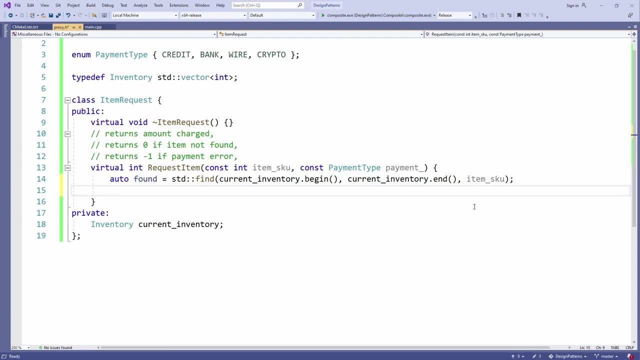 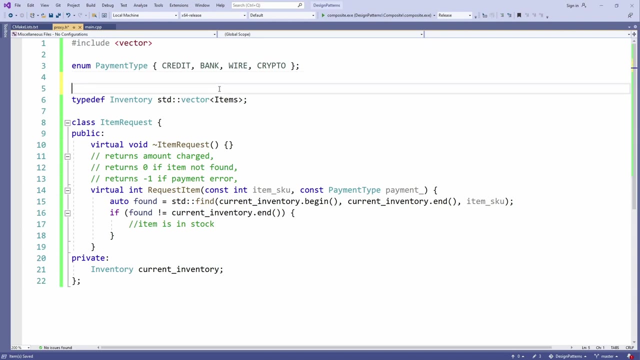 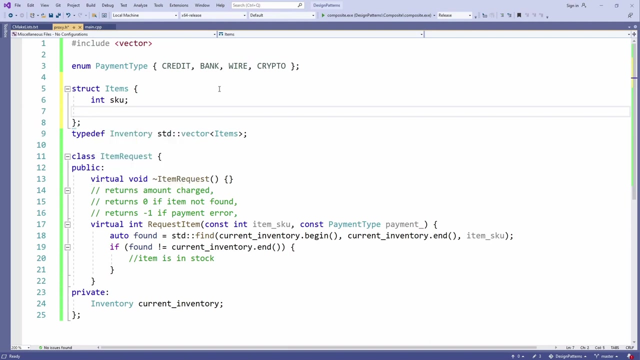 if this is not the end iterator, then we found it. if found is not equal to our inventory item is in stock, let's say so items. it might be better to do items in a way where it's like a skew and we probably want to count of how many are in stock, something like that. 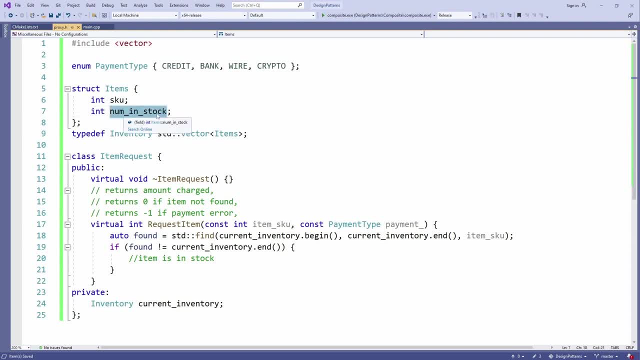 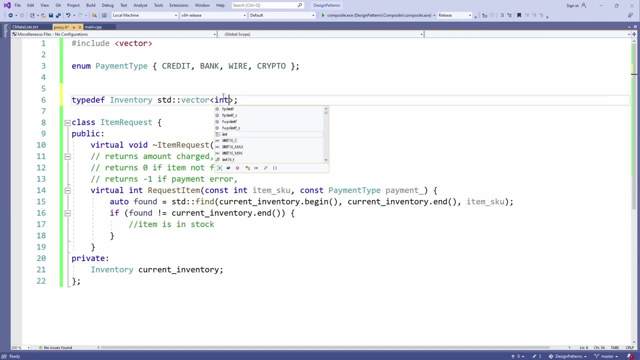 but then we need to think about ways to clean it up, because what if, when it's out of stock, do we remove it from the inventory or do we leave it there with a zero? so maybe that's getting a little, you know, in in the thick of it and you're gonna mess up, for example. 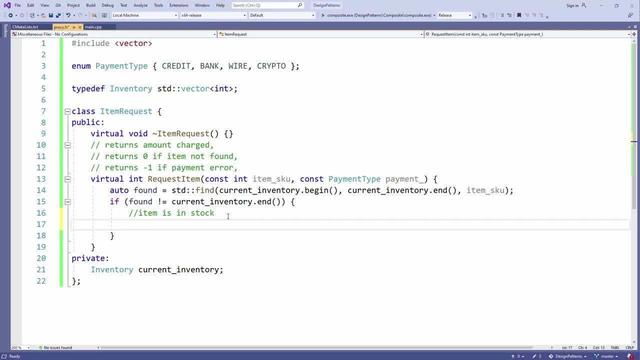 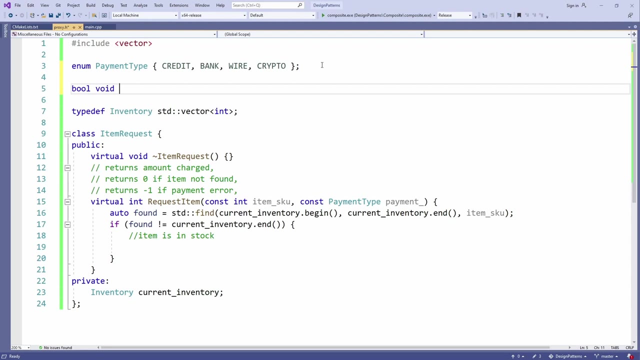 but if it's in stock, we would check the paper. if so, we need something here that would talk to the uh, the end too. uh, let's just make a function to sudo that up. so we would go: boy, oh, i guess items need a price too, don't they? okay, i'll get this sorted out. we'll make a proper. 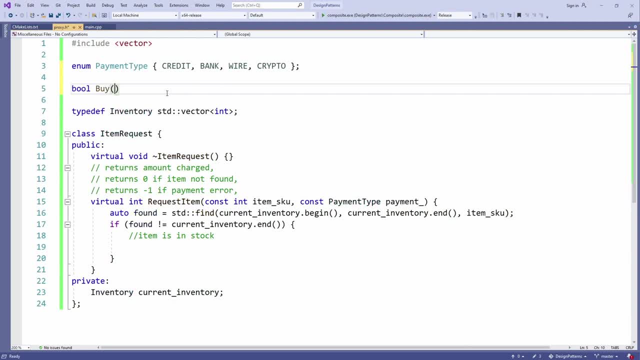 we're gonna have to skip over a lot of details because, well, reality of this example is it's got to be simplified, so it's going to get way too complicated if i add every possibility and check every angle. but it's just an example. uh, let's go charge, so maybe we 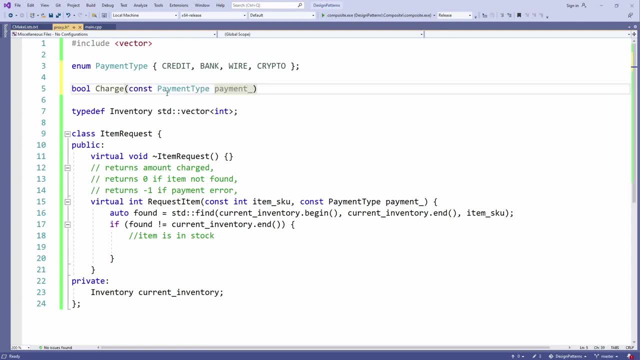 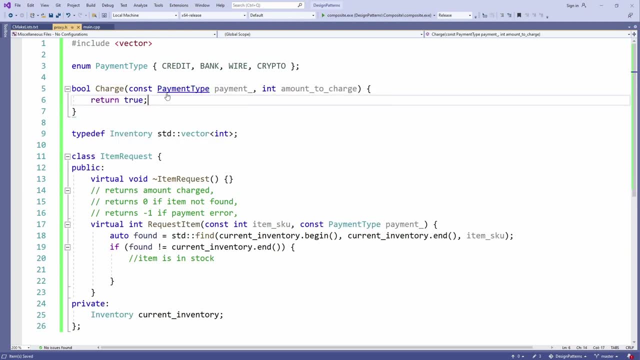 have a function that's called charge takes the payment and, uh, i don't know it's charged for. now we're just going to return through, which assumes we charge the amount from the proper account. now, this payment type you're going to have to think of as being more info, like all the 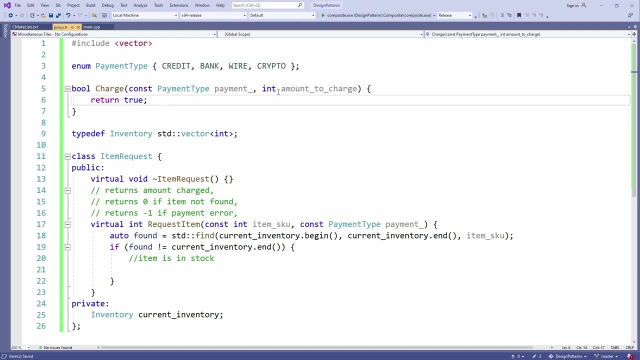 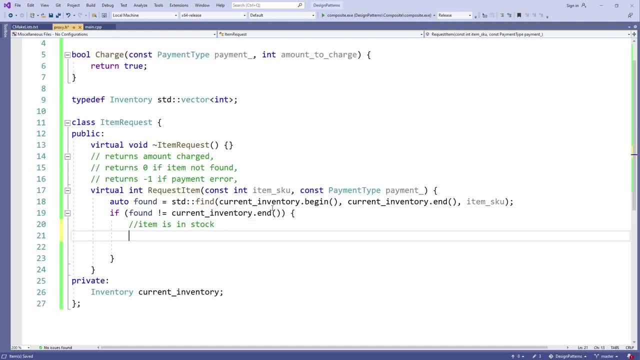 info to do the thing. so maybe it sends requests somewhere else, but for now we're just going to assume that this succeeds no matter what and returns true on the charge. so we would just go: vitamins in stock, try to charge the card. theoretically pass in this payment. 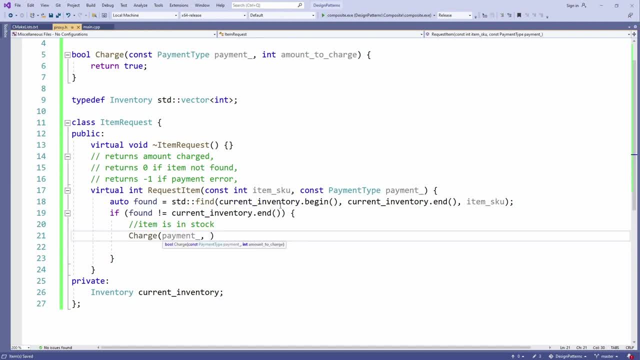 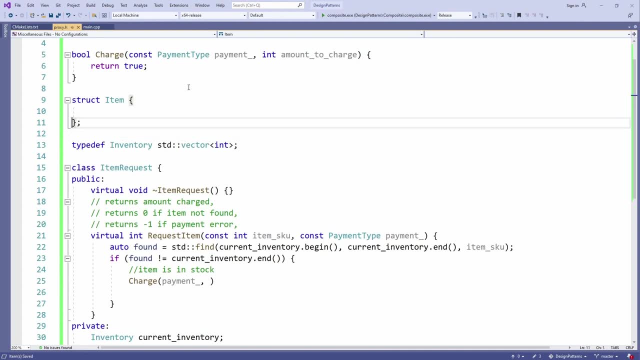 in an amount to charge, and we don't know how much it's going to be, but we would have to check based on on this. so let's work this up. after all, We'll just call it item for sale. That's what this inventory is going to be: a bunch of items for sale. Let's have the SKU. let's. 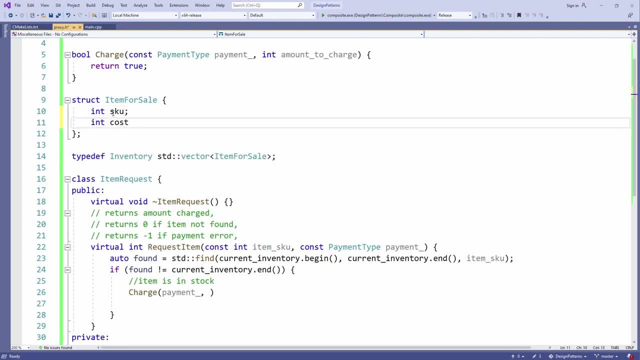 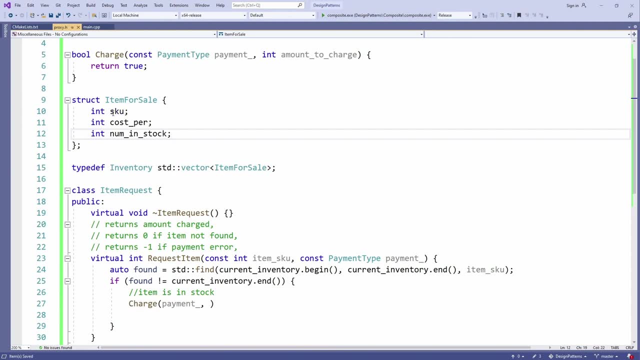 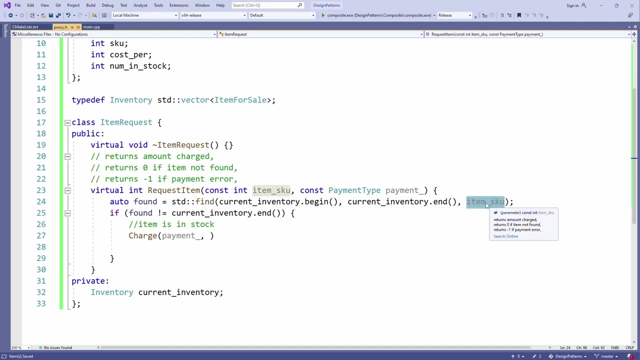 have the cost and let's also have the in stock. That should be good. Now this gets a little trickier because it's a current inventory and we need, instead of just items view here. it's obviously not going to be able to find that, so we're going to have 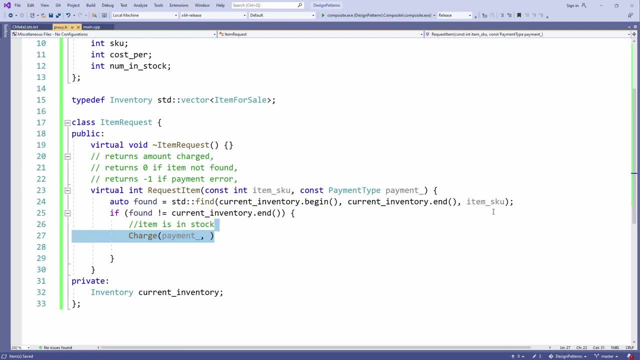 to put something else here. Now, I believe what we can actually do here is put a lambda And basically we just go through the inventory and check: does this allow it? Let me double check. Okay, if we want to do it this way, we have to do find hit in this case. So we 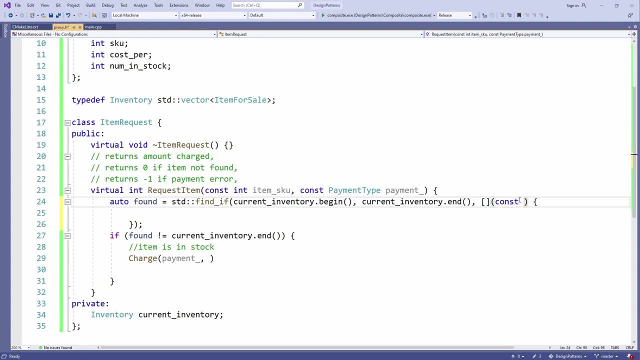 would have to take in an item const, item for sale, just the members of this vector. basically, by reference, We'll just call it i. And now, in the body of this lambda, we're going to say: if i dot SKU equals item SKU and i dot num stock, it's greater than the. 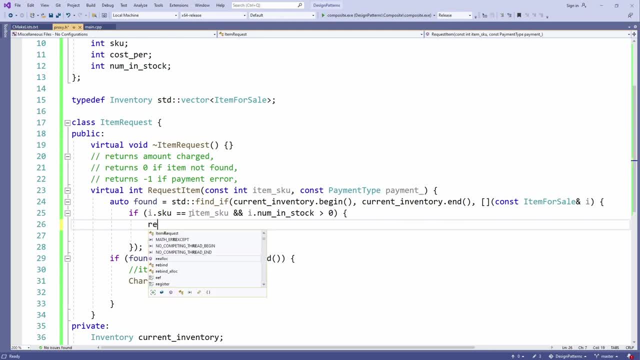 zero And that's the case. we return, And that'll be all we need for the find if code. So it implies that it returns bool. We want to make sure it understands that. We could put that here like so, which is part of the lambda optional syntax. Otherwise, we want: 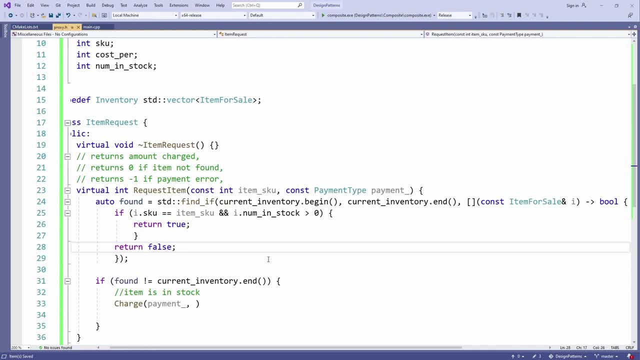 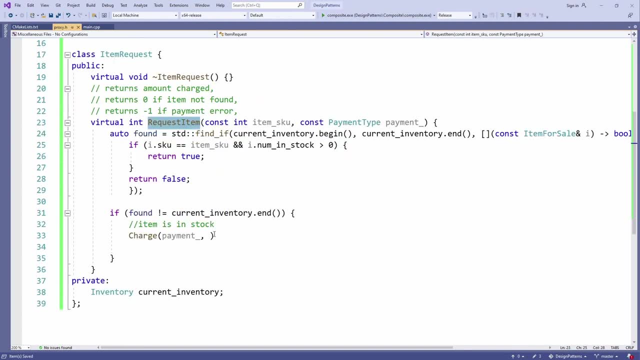 to make sure we actually return false. That's the fall through case here. Okay, so that's the default Rest quest item And you can see that well, found is going to be a little different with find if, because this returns, all of them match. Now we know it should just be one, But the 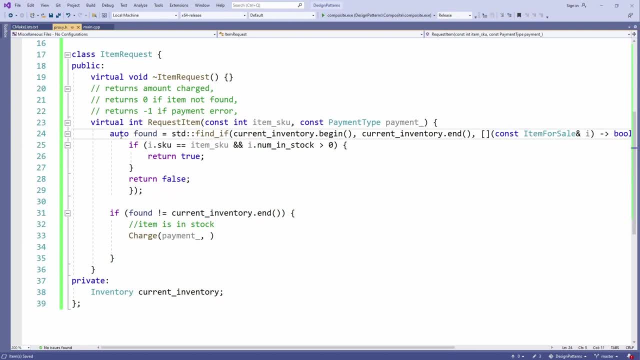 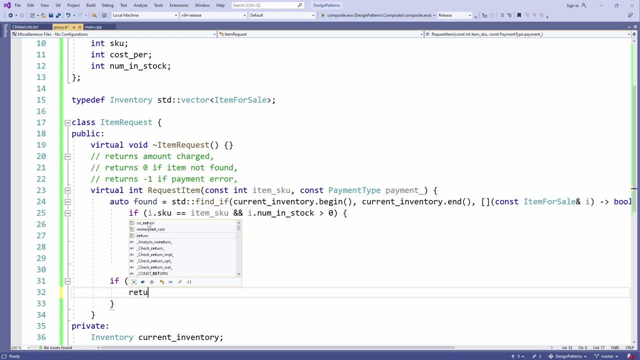 thing is, this is going to be- let's see if it hovers over. Now it's going to be an iterator, So it's going to be a little bit different. Let's go ahead and just make sure this compiles. Okay, so if the item is found, we essentially want to return the amount charged, So that's. 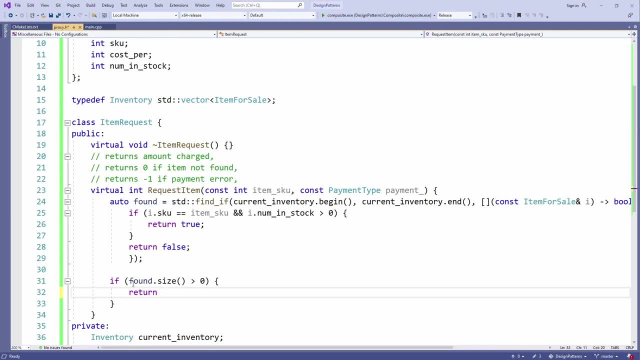 all we would do. If found is greater than zero, it means we found an item in stock. Now find if can make quite a large array or list or whatever you're working with a vector, But in our case there should only ever be one match and one item in stock We could. 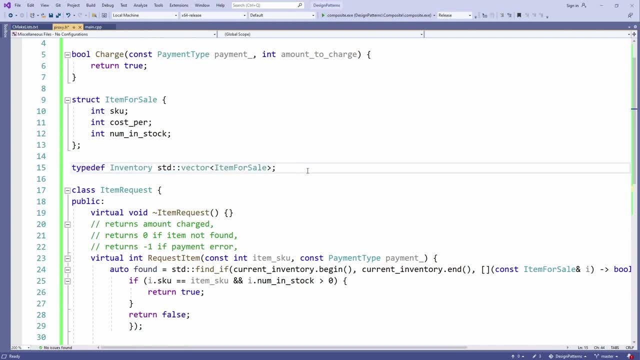 make more sure of that with better management of how this works. But we're kind of overlooking that Because you know, technically we can make a bunch of items with the same skew. This should be unique, So we probably have something to make. 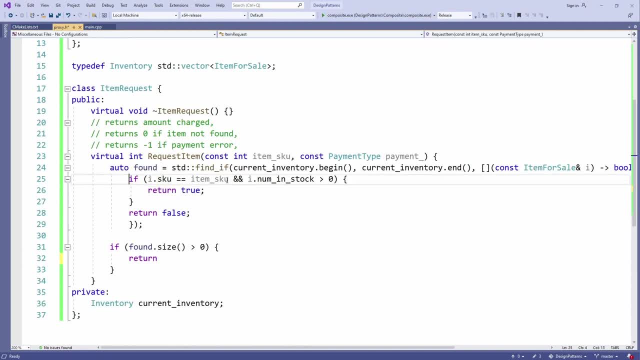 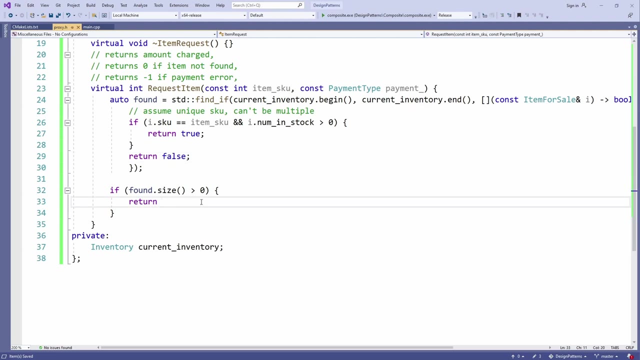 sure that's unique, So just assume that maybe we will even put that in here. Assume unique skew and be multiple, All right. well, it's just an assumption we'll make, even though it doesn't quite fit the data type correctly. But let's just continue. So found at size. 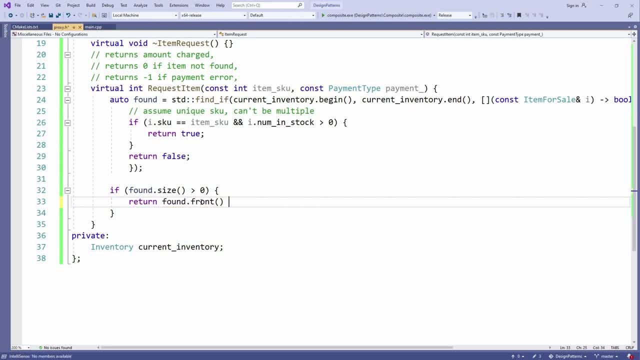 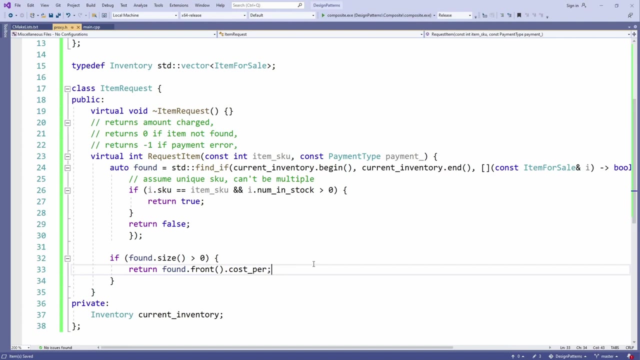 greater than zero. So we assume that the one in the front is the one. So we've returned cost per. This only requests a single item. I guess you'd have to call it a bunch of times to keep getting the same thing. And once the amount is charged we want to produce the count of that. So actually, 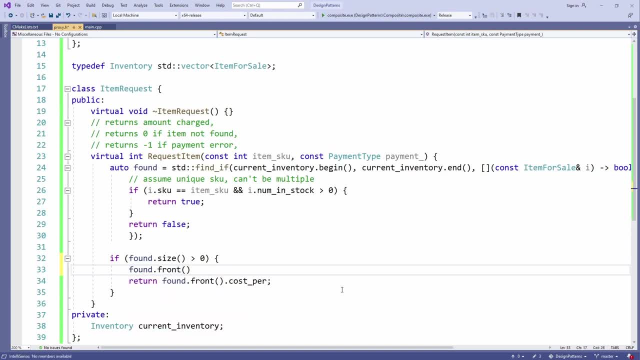 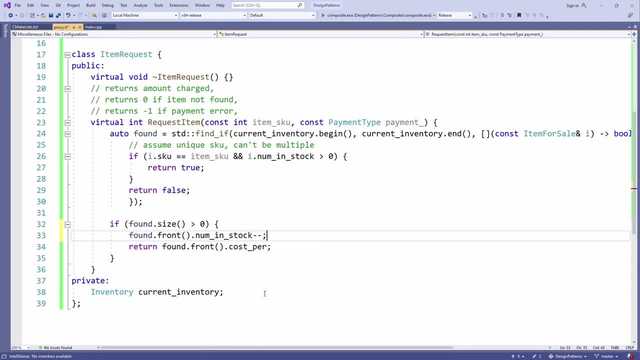 we do foundfrontnumInStock. Okay, Minus, minus. So there we go. That would reduce the number in stock. However, it won't actually, Because this is just a copy, It's not a real inventory, So that's not exactly going to. 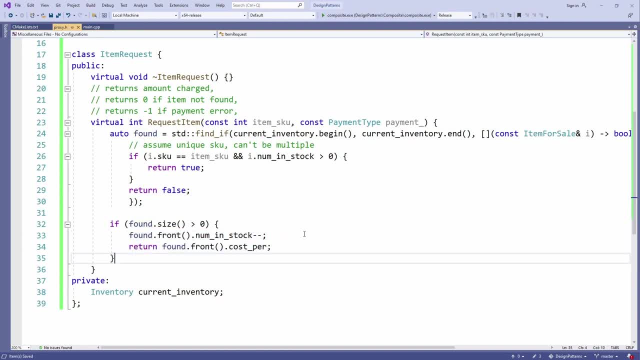 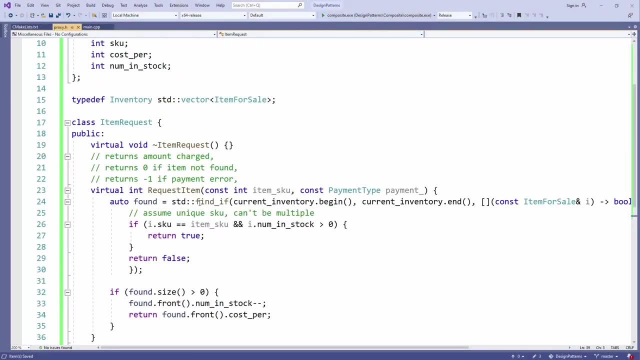 work like we think it will. This return is fine. If we want to actually reduce the front, we might need to Use other methods. For me personally, this whole find if kind of complicates the whole thing, So I'm going to just rewrite this in a better way that I like better. So, essentially, we just want 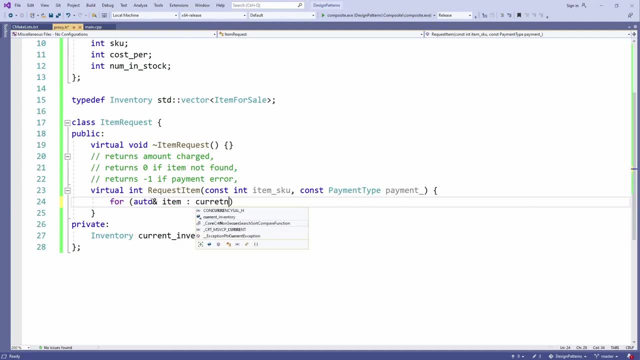 to go through the inventory. So let's just do that. So let's just make a auto reference to an item, Go through the inventory, And this is going to simplify a lot because we can just do the direct check Item dot skew. 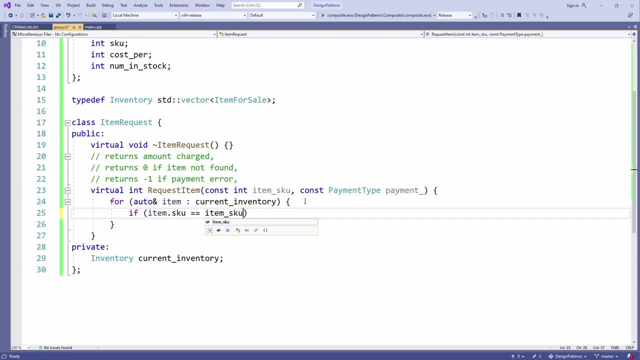 If it equals Item skew And item dot, NumInStock, And we return the itemcostPer. And if it goes all the way through this loop without returning the costPer, Well, let's make sure to reduce it. So this minus minus will work, because 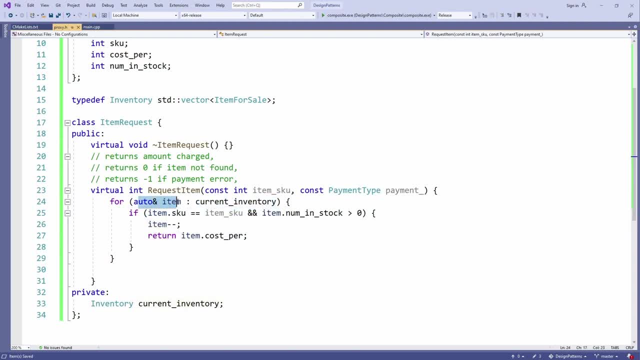 It's a reference to this current inventory, So that will work properly. And then we'll return that and we're good to go. Next time you go to check, it's possible that the numInStock is no longer greater than zero, and it won't. 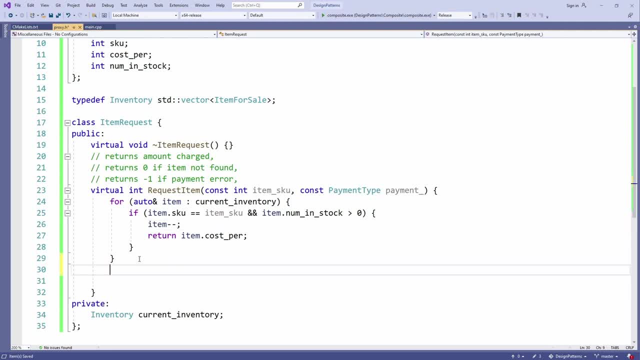 find it. So that's an interesting thing. So we can return zero if item not found. That would be like: right after this We don't have the charge We need to charge, right, So we would do that before subtracting. 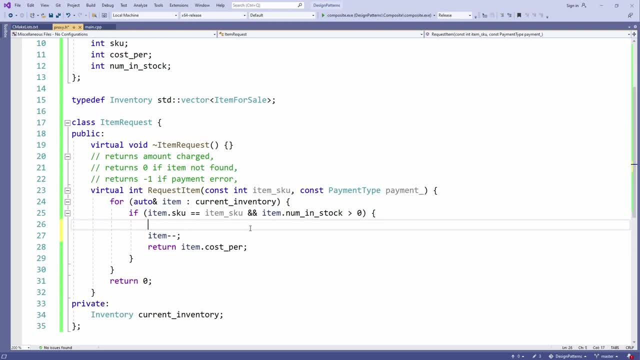 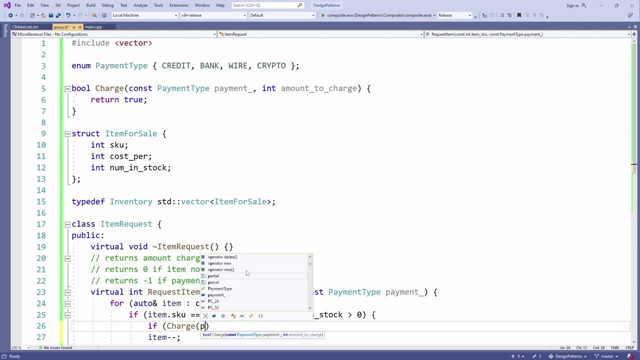 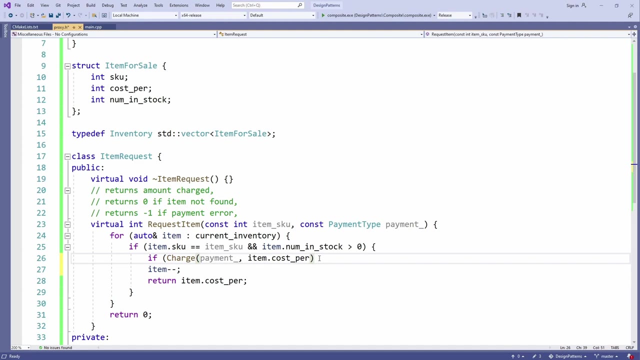 The item. So if we find the item, it's in stock and we attempt to charge. So let's just go. if Charge, We need the payment passed in and the amount to charge, which is going to be this itemcostPer. 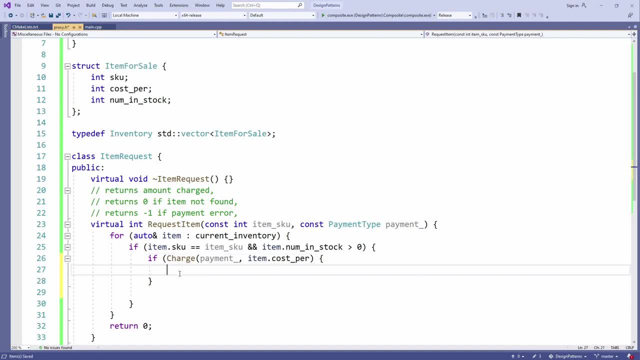 So if this returns true, then we return all this stuff and say the charge went through, Subtract the item, Tell them how much we charged them And if it doesn't go through, so it finds the item and in stock, this charge fails. 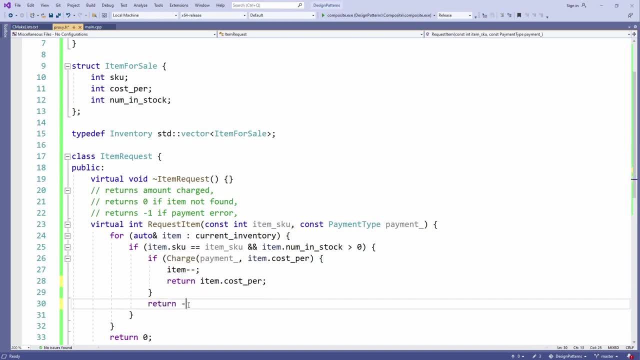 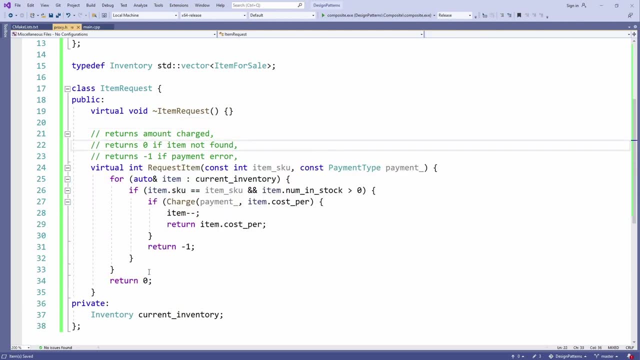 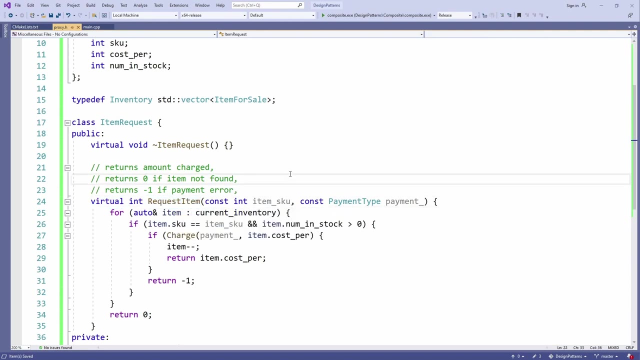 We want to return negative one as a payment error. So there's our base request item. It should work pretty well. So this is an interface class, but it's not a pure virtual interface class. Since we've defined request item, you could do in a pure virtual way if you want. 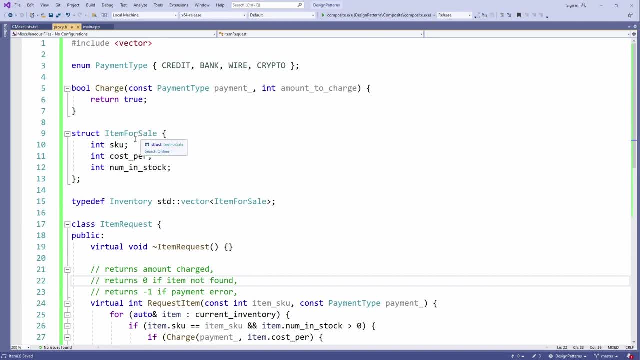 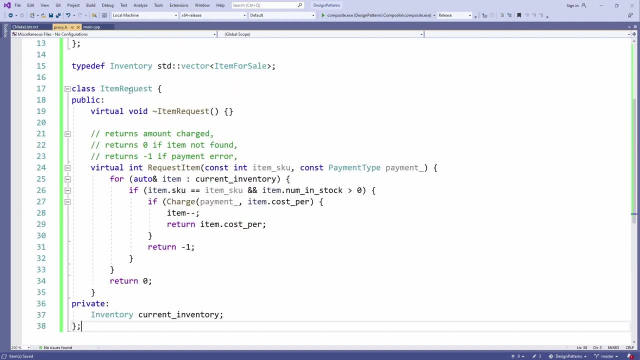 I'll leave that to you If you want. There's a lot of examples up there often do it that way, but I don't find it to be necessary for this more simple example, All right. So we've essentially got a thing we can use in our main, and this is the real item. 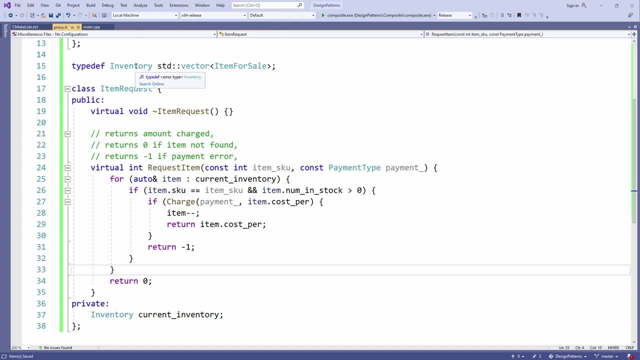 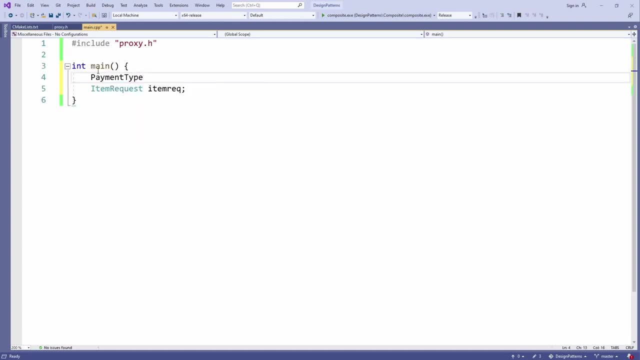 What we're going to do now is put a proxy in front of it, So let's just test out the real one first, just to make sure it actually works. So we need a payment type: Our payment, Our payment, Our payment, Our. 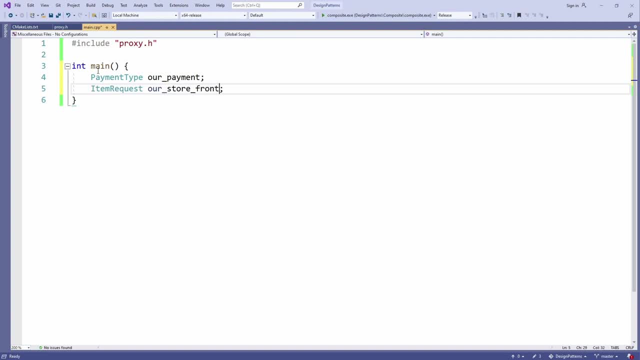 Let's call this storefront Payment storefront. All right, Payment, And we need our payment to well. I guess we could be whatever we want to be. Let's just do a credit card right now. So then we just go our well. we need to populate the storefront. 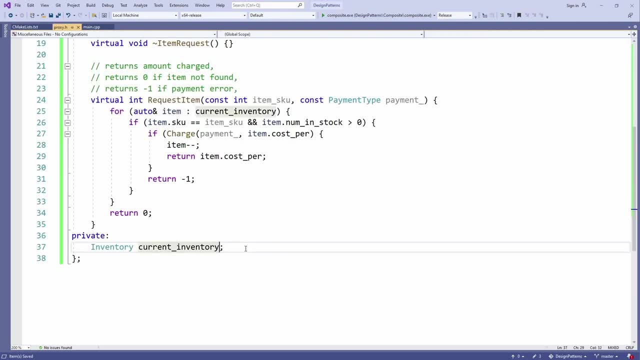 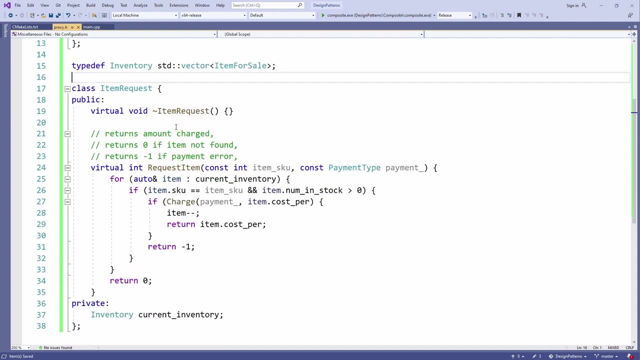 It doesn't have anything in it, As you can tell. we could have it. Give it that base instantiation of some stuff. Right now it's just going to be no items actually for sale, So maybe we want in here and add inventory type of thing as well. 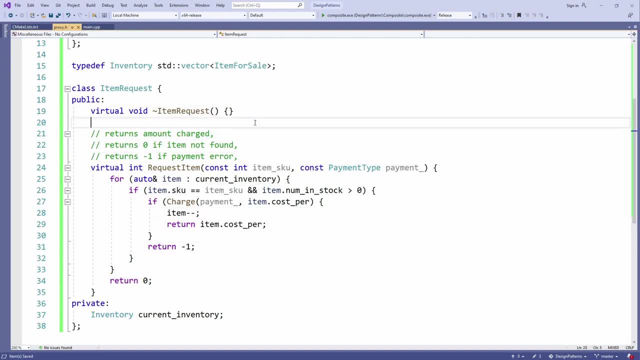 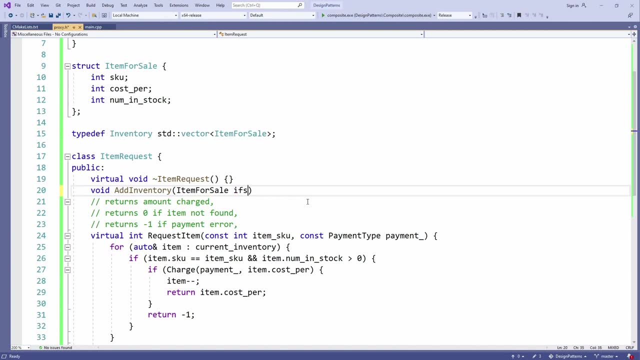 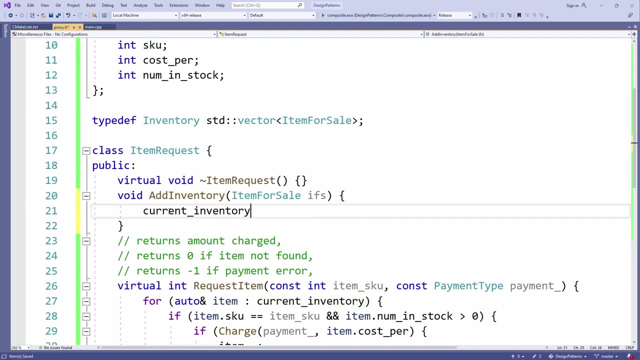 But we've been a bit naive and haven't added that. Let's just do it, I guess: add inventory And we'll just take in items for sale, and we could define this as just exactly what you think: Current inventory- Pushback. 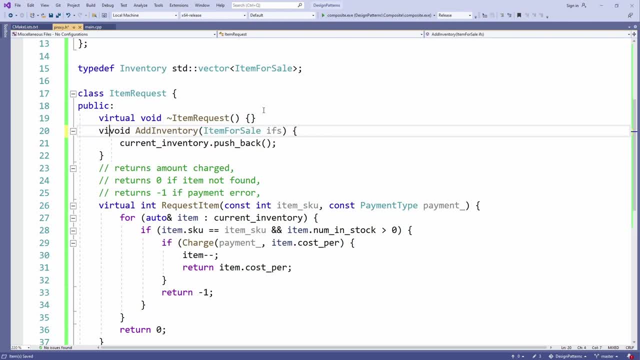 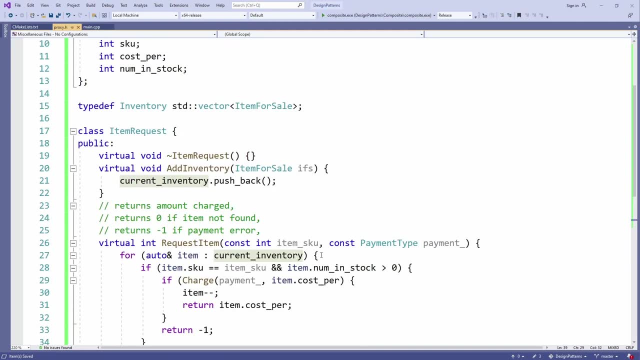 All right For sale. We could make this virtual in case they want to override it as well. We're doing that. We probably want to make this protected rather than private. That way, if you're inheriting, you can still write functionality around current inventory. 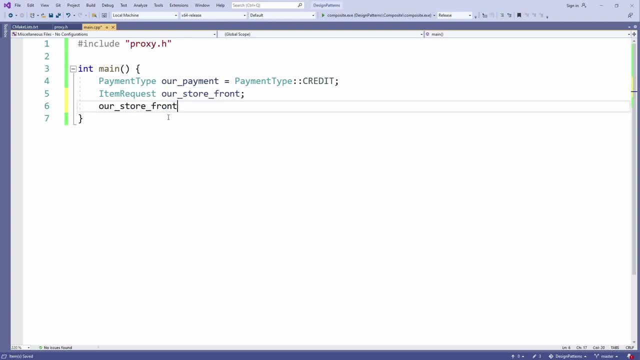 And there we go. So now we can just pass in a few items here, or something like this, Was it? It was skewed Correct Cost and number of stocks: View Cost, Number and stock. Now is it going to like that? we have instantiated this inline. 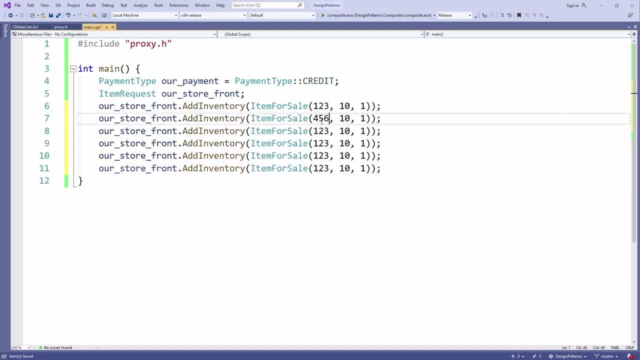 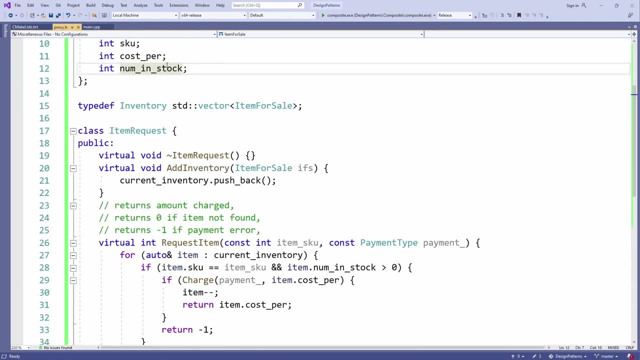 I don't know. It might confuse it a bit. Let's just put in a couple of things here. So it kind of makes sense that we let things stay in inventory with zero in stock, because that would kind of give us a flag to replenish. 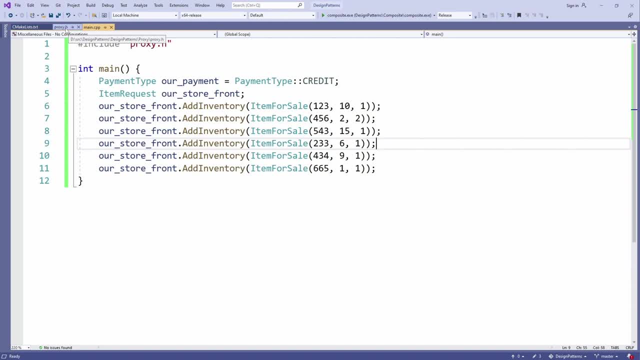 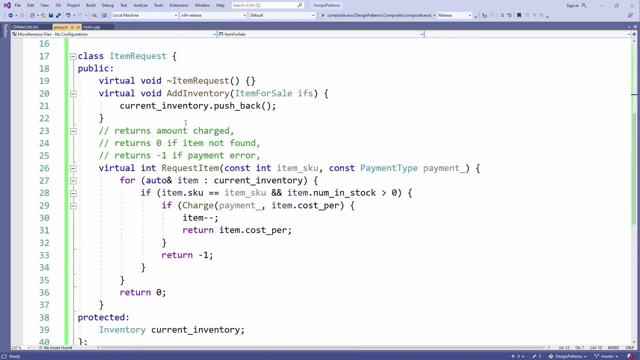 Something runs out. We try to get more Type of thing, But that's for a later setup. Let's see if this code actually works And you actually push this back. So the thing to do currently would you know if you try to add inventory? we got to think. 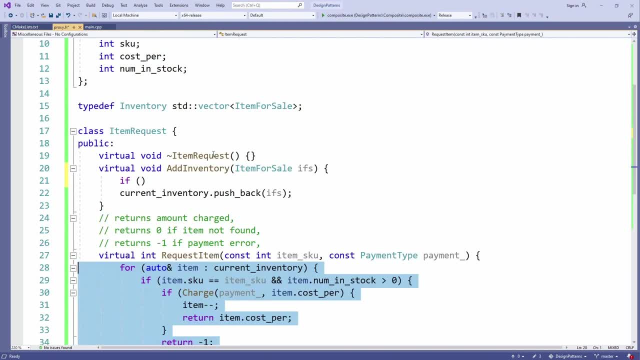 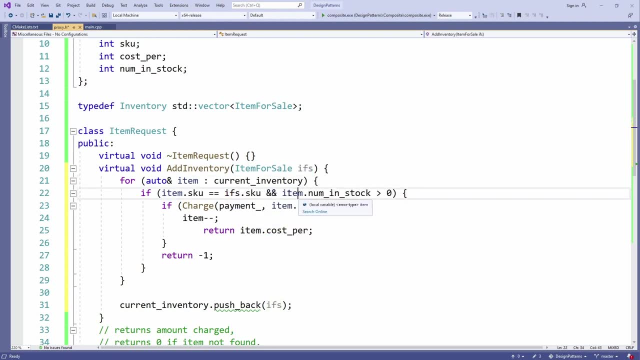 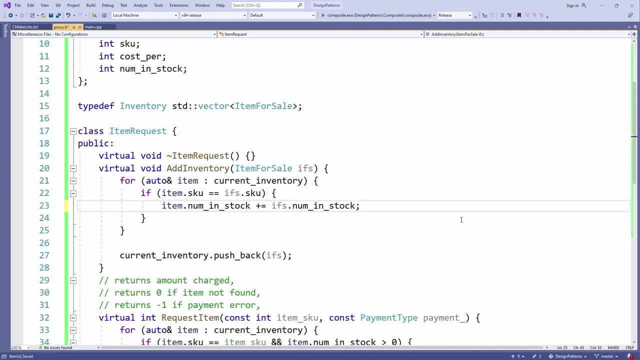 about this a little bit. If it already exists, So let's take this same code here, Go through all the items, See if it matches This new item item skew. if it does, we would just add that to the inventory with a plus equals, so we could just do. 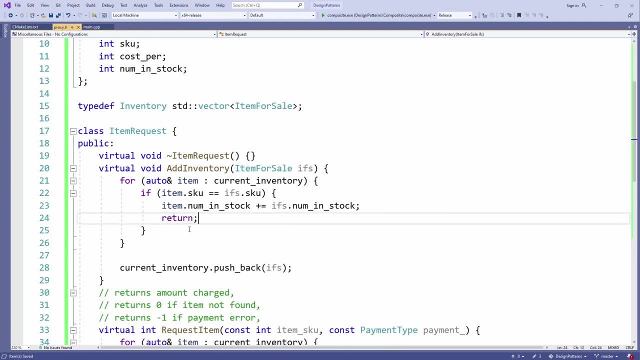 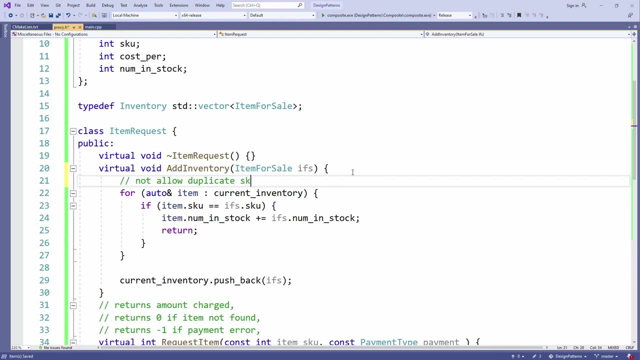 that and of course, if this happens, we want to be sure to return, not push back the new one. so this would be not allow duplicate skews. instead add to known stock. so there we go. so if it goes through all this and doesn't find a duplicate, then it just pushes back a new one. it's a pretty fine. 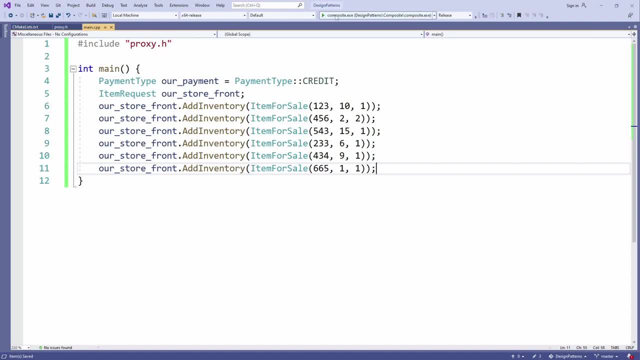 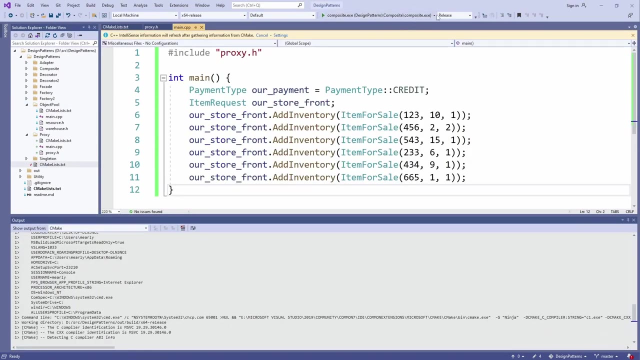 add inventory request there. so let's just go ahead and make sure this runs. i'm going to switch this to proxy. where's proxy? i don't see it. oh, we need to add it to one more cmake here the level above it. sure to add proxy here now. it should show up as soon as this is done. 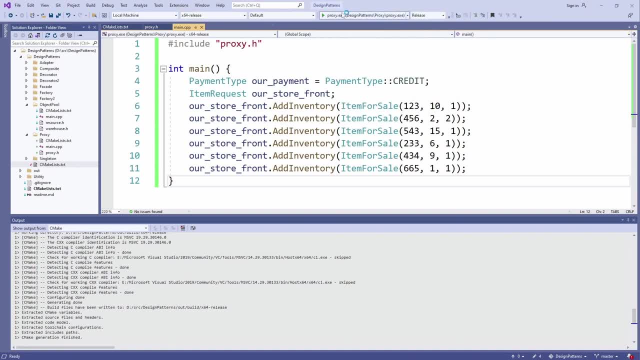 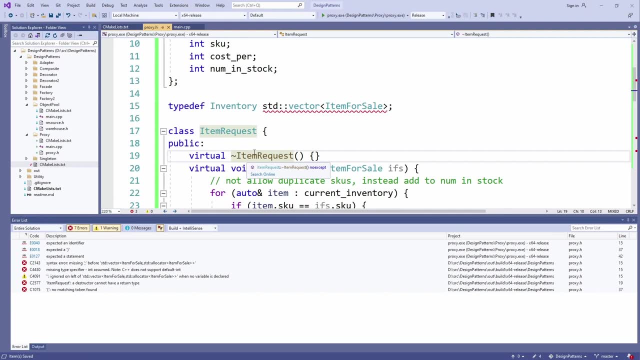 there, it is okay and let's just hit play and make sure everything's okay. and let's just hit play and make sure everything's okay. and let's just hit play and make sure everything's succeeds. we have an error? um, okay, there's that. can't have a return type on a destructor. 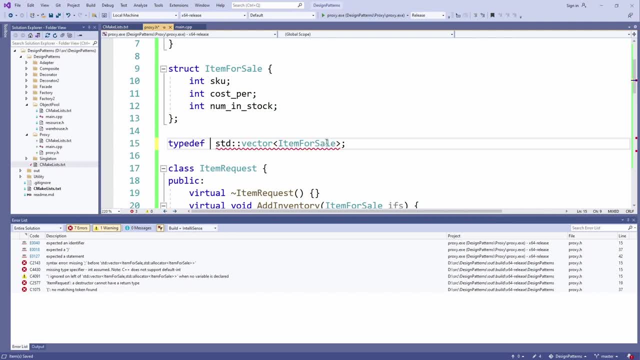 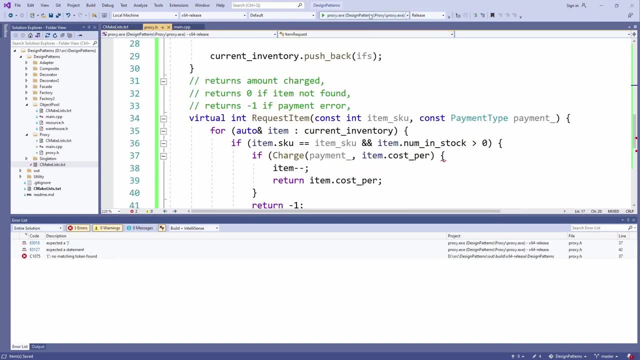 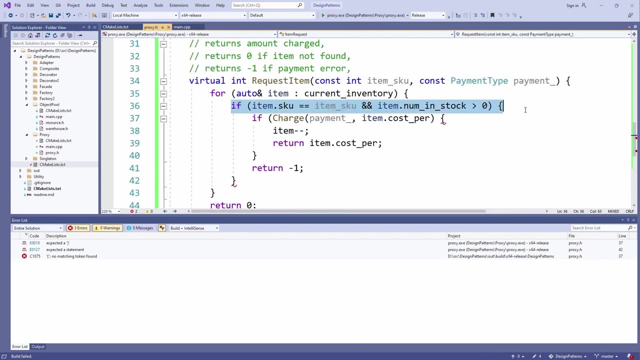 am i doing this type def wrong? i think i am. i think i have reversed. i think it's like that we say: this item for sale is called inventory. let's try that now. okay, i think this is okay. let's say complain about that. so we got an if statement here, statement: oh, this item, we need a. 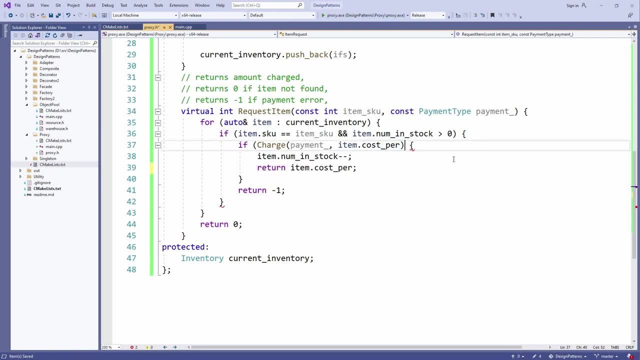 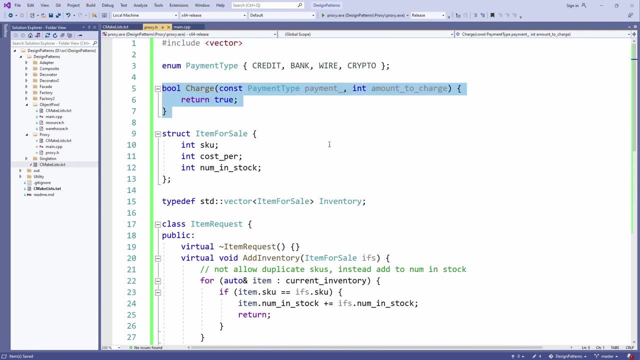 number in stock here minus minus, and we need another parentheses there. so this returns the charge, right, okay, yeah, that was it, because this returns a boolean. in our case it's always true because, you know, we haven't implemented a true payment system, so we're just assuming the payment works. but we do. 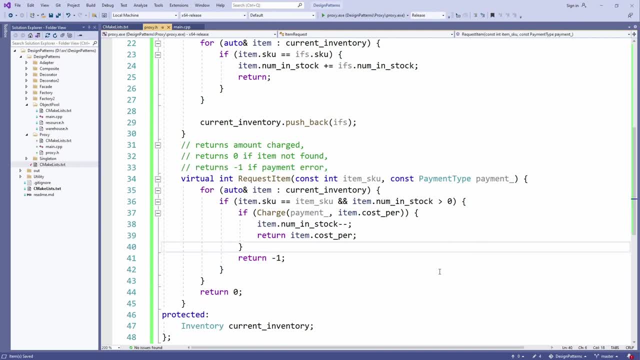 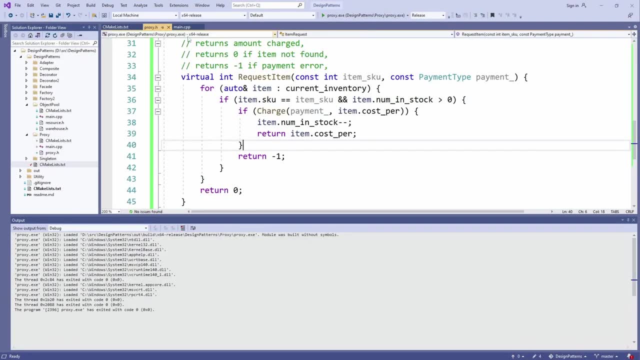 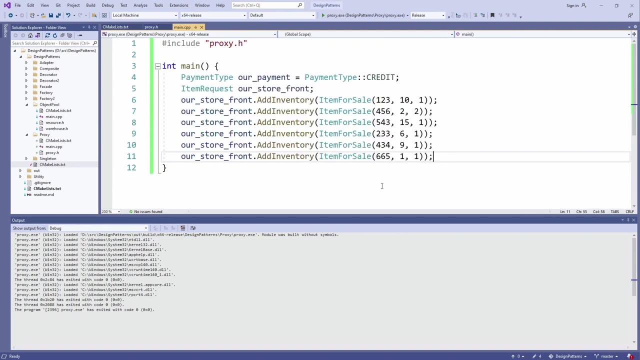 have way in case it fails to return payment error. so that's, uh, something we could do later if we want. that's getting into the real world, so we're not going to go there. okay, it all compiles and looks fine, so you can kind of use this, you can request items, so you got all this storefront. 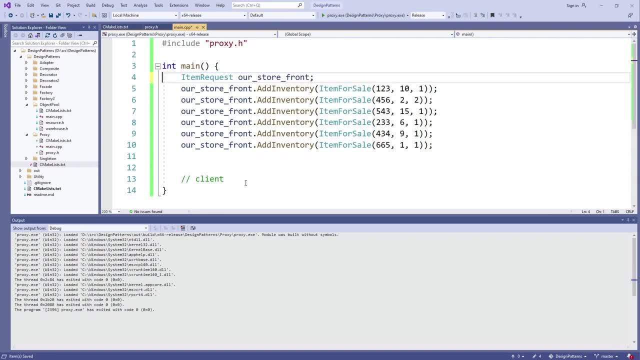 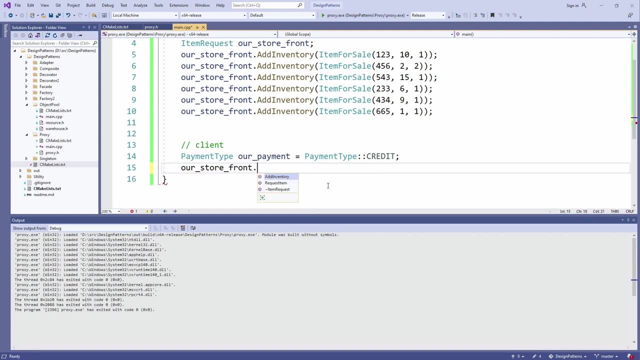 now we're in client world, so you would want to, uh, just basically do stuff like our storefront dot request item and we'll have a return code here. make it auto for now. and what item do we request? i don't know. we need a skew, so we'll put in some random numbers and then we want our payment to be passed here as well. 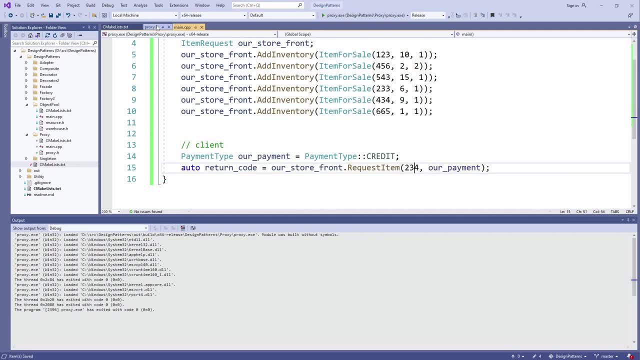 in details. you know, if we're really going further with this, we could say shipping, detail, all that stuff. but maybe that would be a great proxy actually to put the shipping on that. because that's essentially essentially what you do with proxies is you usually add, add some additional stuff to whatever it was before. let's go ahead and display our output here. 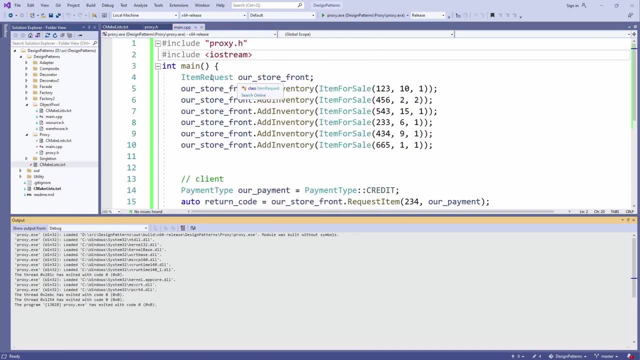 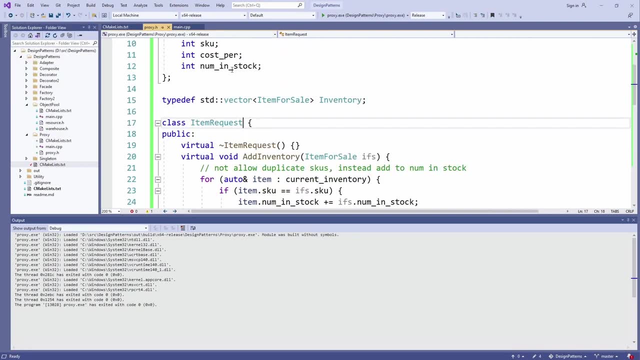 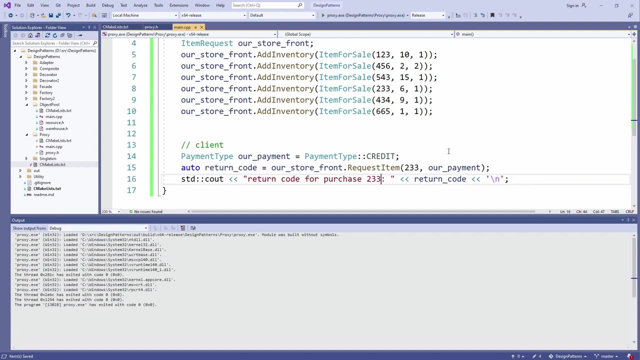 and we get code zero. what is code zero? well, we can take a look at it and say: item not found. okay, interesting. yep, that actually makes sense. there is no two, three, four in here, but if we look for two, three, three item, let's see what happens. actually, let's just, uh, copy all this. 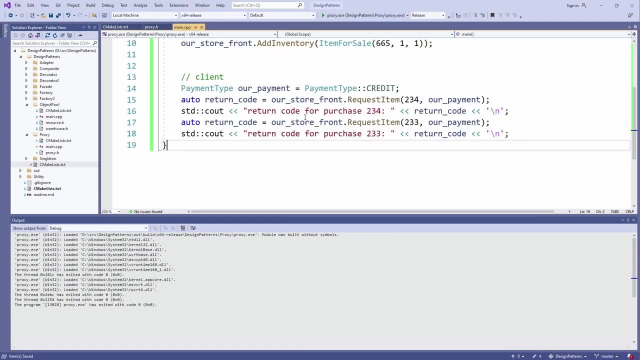 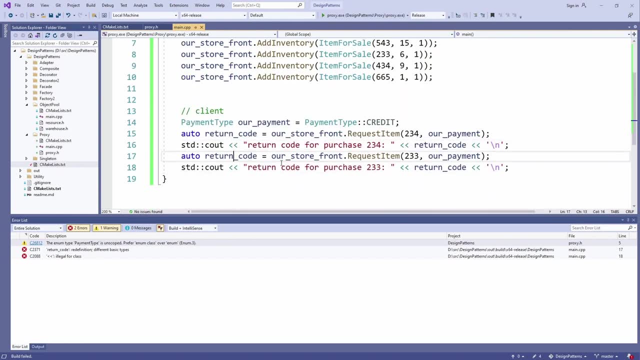 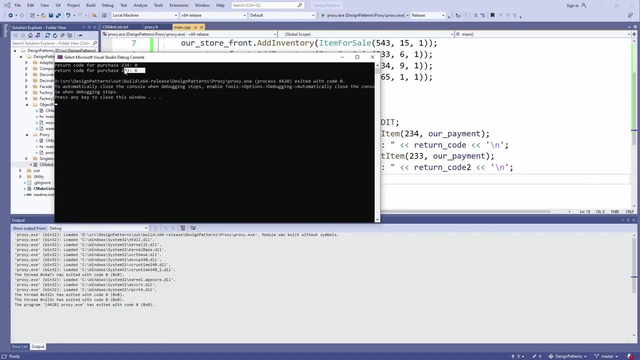 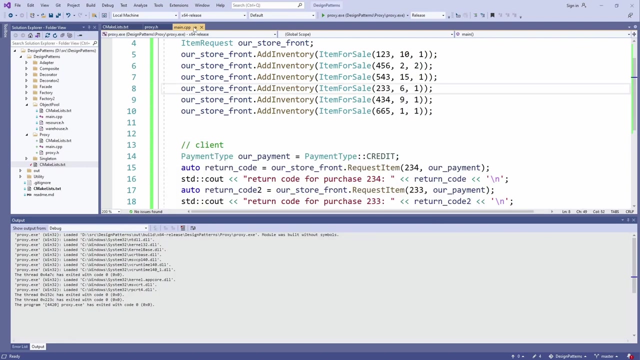 code down and let's say plugin, it is: oh, we're saying return code twice. let's go like that, okay? so for the first one we got a zero or item not found. the second one we got a six, which is the cost. there's the cost, so that works perfectly, okay. so if we take it a step further and make a 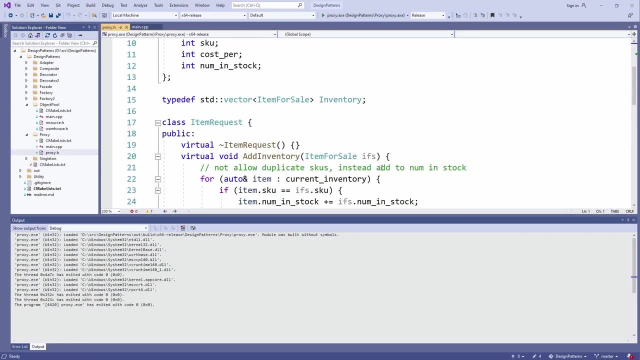 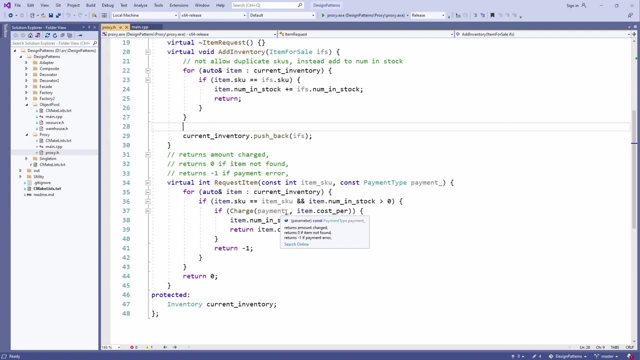 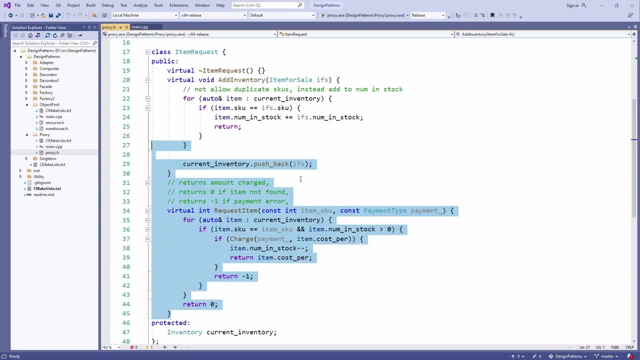 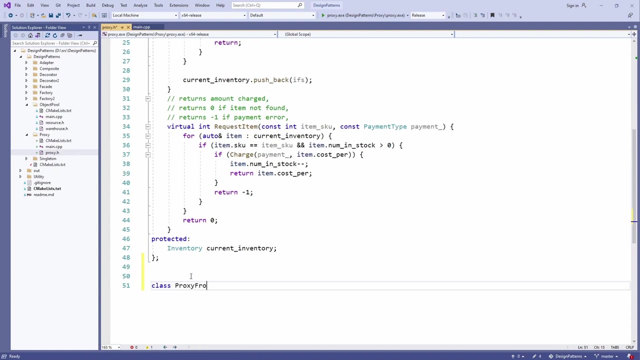 proxy so we can do some special stuff. so, while our current item request works fine, what we could do is: uh, we could say, we'll put another front on it so that we can gather shipping before we request the item. so what we do is we just go class um proxy or address and we will take in. 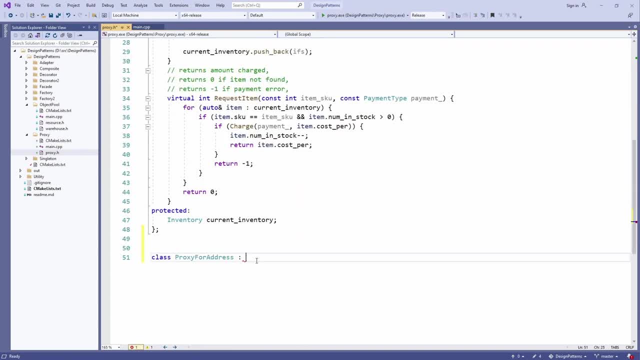 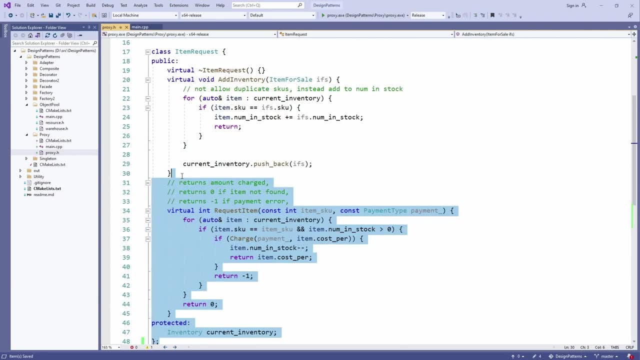 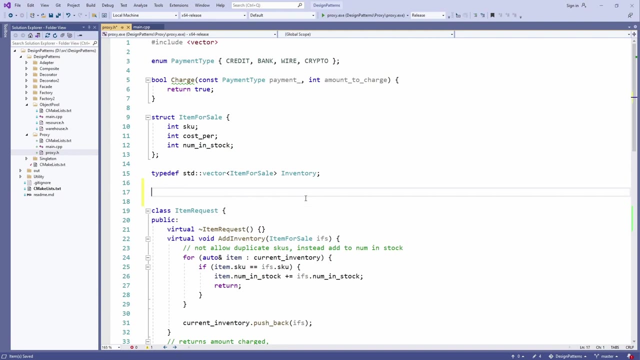 or we are going to include this item request here as part of this class. now, if this were a pure virtual interface class, we would want to hold a pointer to it. uh, let's actually just real quick, make that base interface. let's just call it a request, all right. 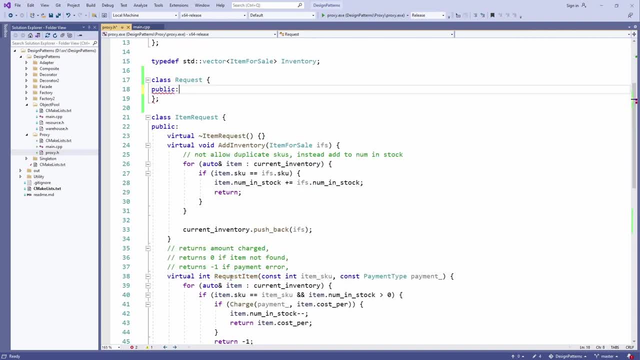 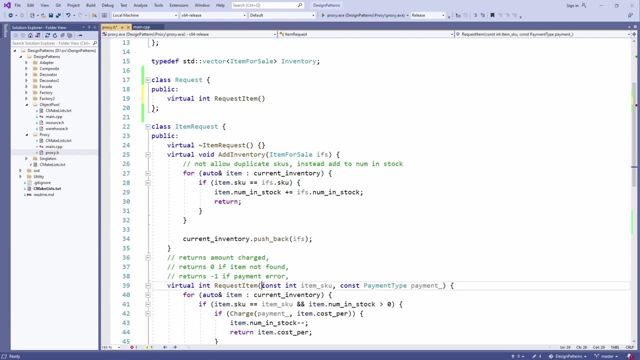 and in here. this is where we're going to have this virtual add inventory as well, so we could put that in here and make that equal zero, zero. all the same stuff here. this time it's going to be equal zero, so that way i have to implement it in this item request. 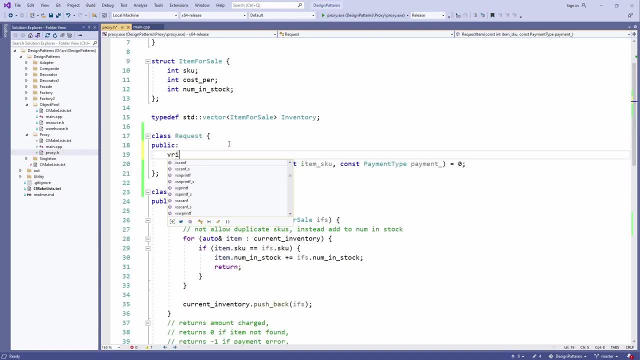 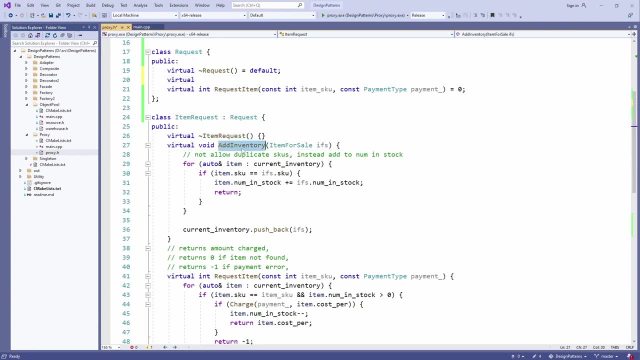 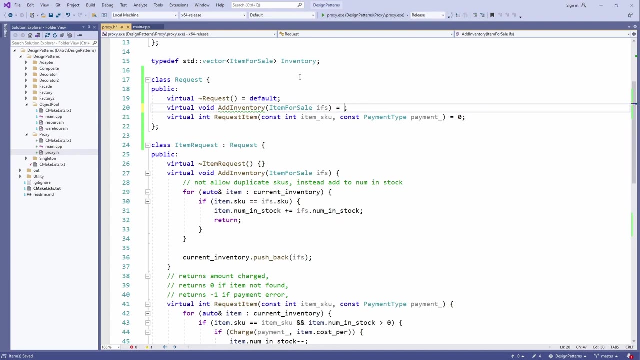 and we do need the destructor here too. there is a virtual add inventory as well, so we could put that in here and make that equal zero zero and make that equal zero zero two. so now we have an interface that can't be instantiated on its own. it has to be overridden. 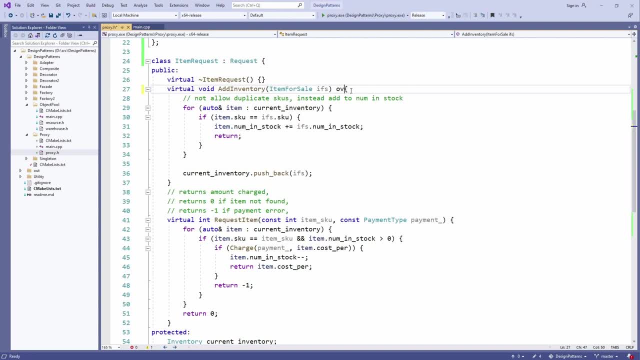 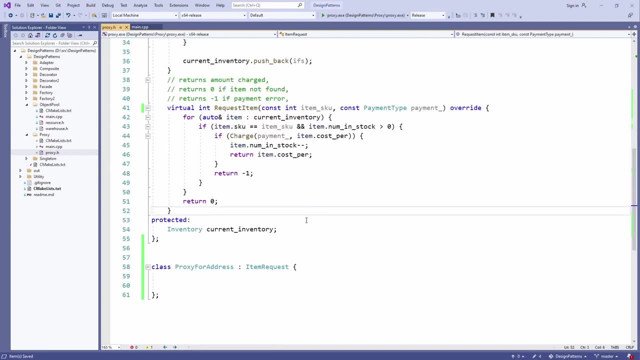 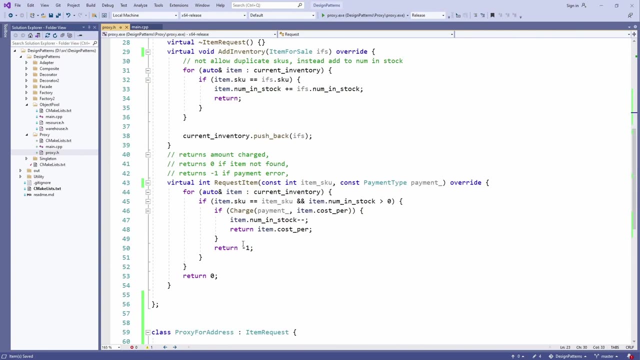 and all these virtuals declared with override. i don't think we need virtual over here on the left side, but i'm going to leave it to see if compiler complains. now this inventory could probably go up to here. yeah, and that would be fine. so there we go. now we've got an actual interface. 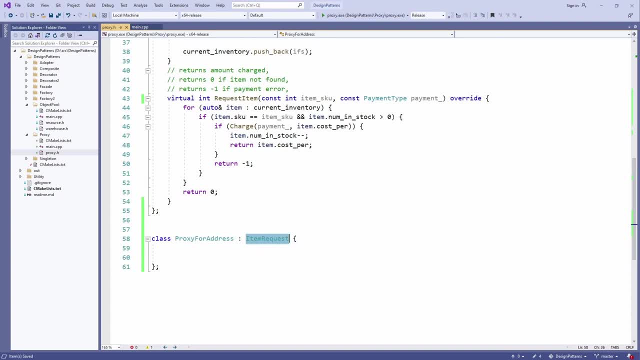 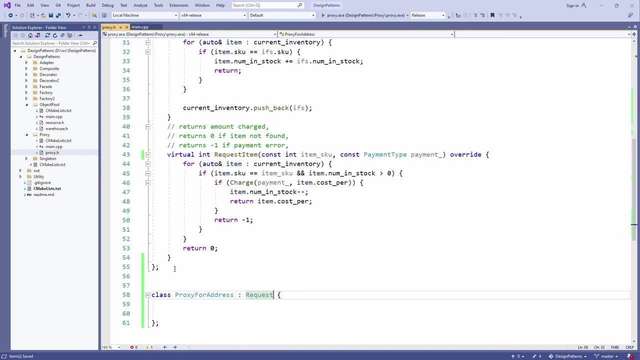 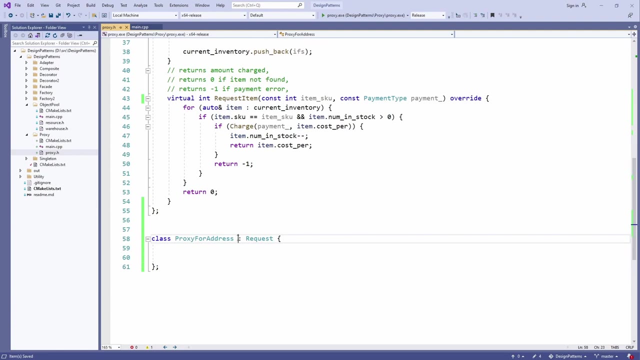 so in this case, what we would do here- so we call this one just- is this interface here. let's make a proxy. let's make a proxy of the item request. so here's the proxy for address on request. um, i want to make this descriptive and long. 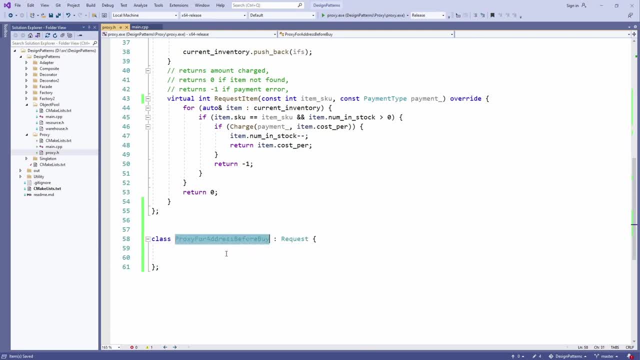 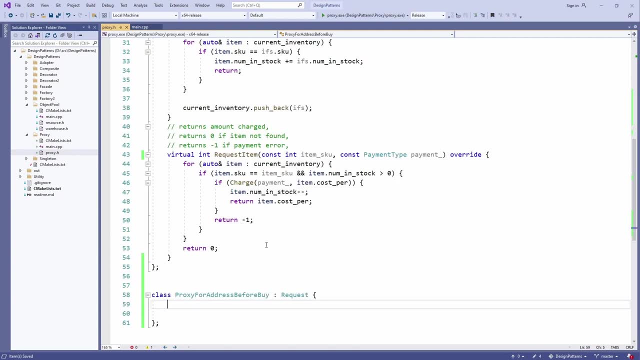 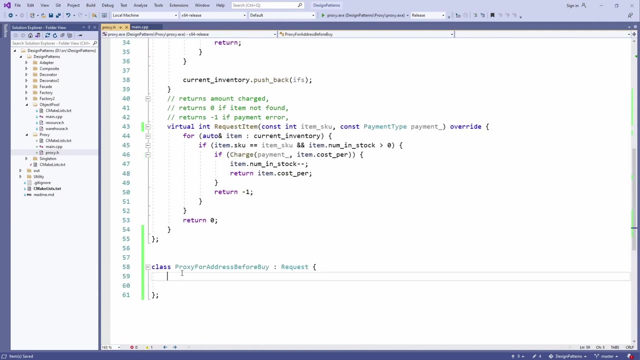 proxy for address before buy: okay, super long last name, but just just roll with it, it's, it's fine. just want to make it clear. so in this we already got all this request stuff, but of course it needs overridden, or so you would think. but we can make a private member here. that is called. 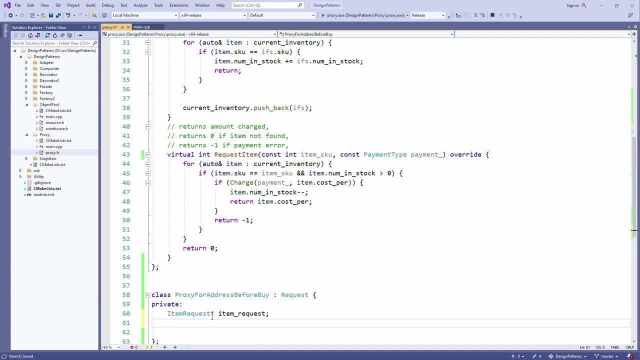 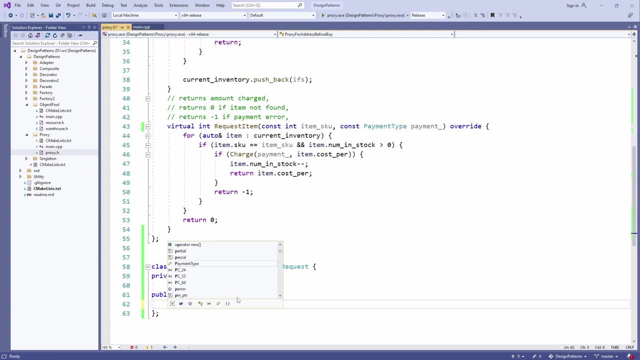 item request: make a plumber, all right, and then publicly we're going to have to have the constructor so that we can set this, and it would look something like this: uh, proxy, yeah, this whole name, constructor, and we want to put in this item like: so, let's call it uh. 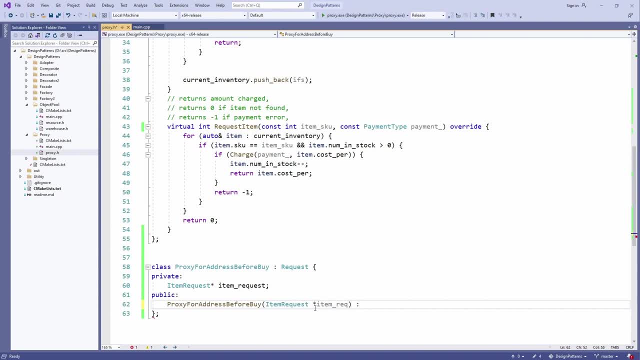 hide, all right. and then we want to just instantiate this. so just do new right, pass this pointer, all right, we're going to dereference it like that and we're going to put brackets over here for anything else, but that should be fine. but that should be fine. 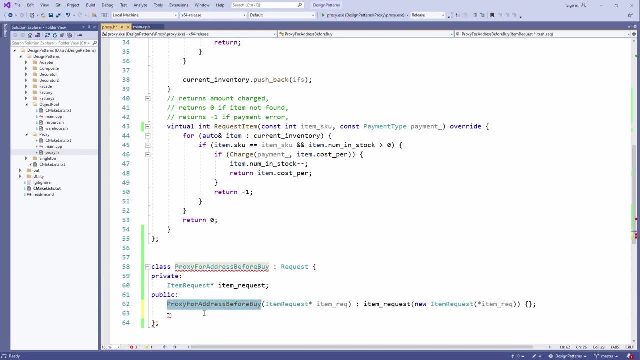 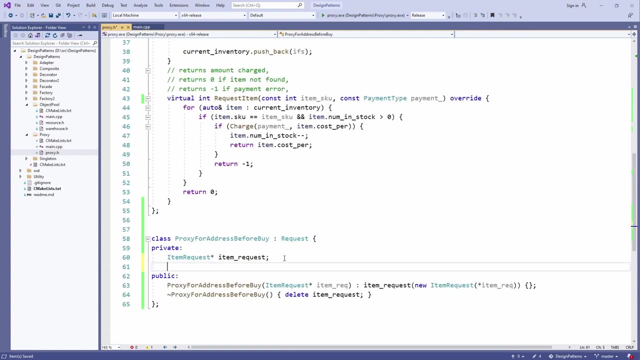 all right then we want of course a destructor publicly here that just deletes the item you have request just should be mostly ready to go so we can add in some more private stuff here. uh, that we want to do because we already know that this item request is going to. 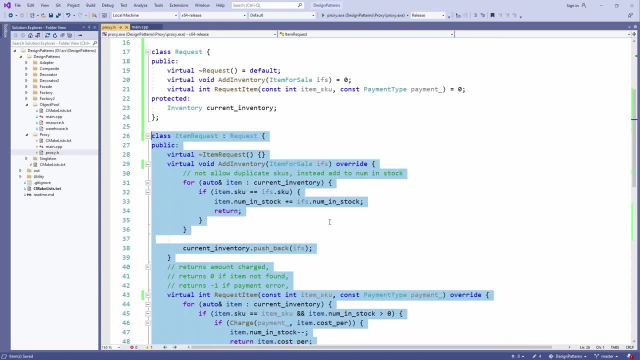 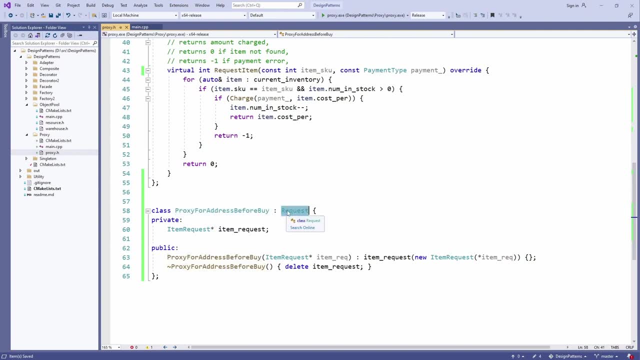 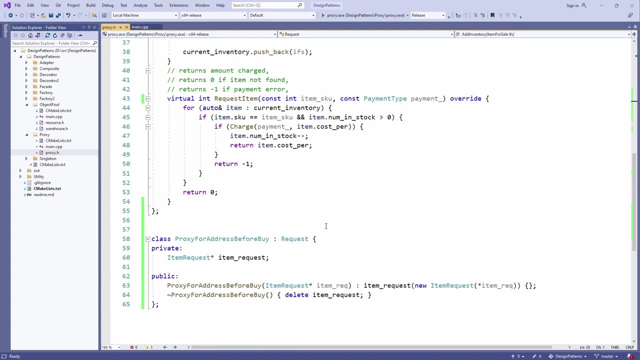 have this whole instantiation here, but now, since this proxitory proxy for address implements this request, we also have to implement these still, which is actually okay, But it also means that this can stand in in this interface. So, rather than the old item request, now we can put a proxy on top of it. So I'll go ahead and 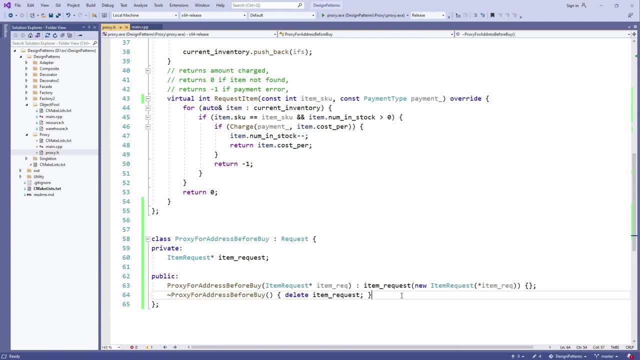 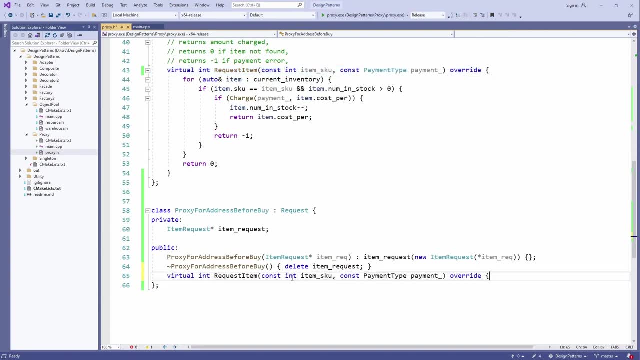 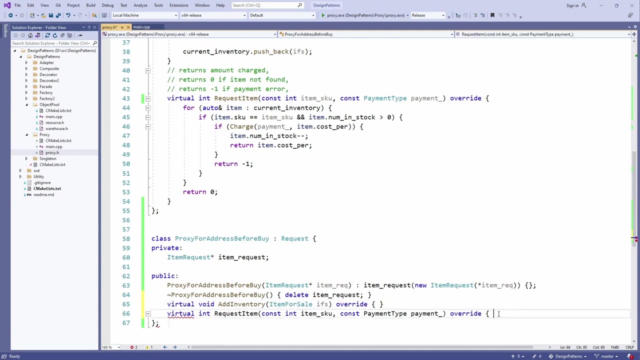 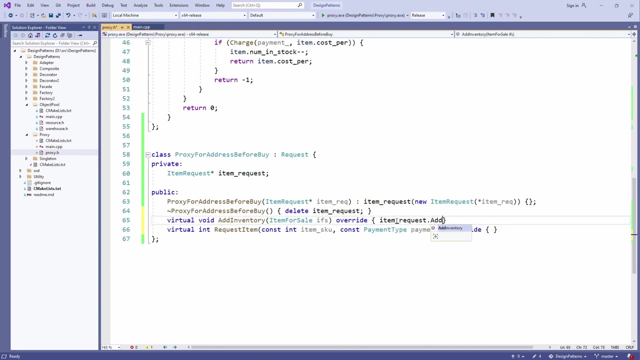 show that. So first of all, we need to implement a few more methods here, like basically all of these And these overridden ones we also need to override. But rather than call everything we've already called and rewrite this sort of thing, just do it like this, Just push. 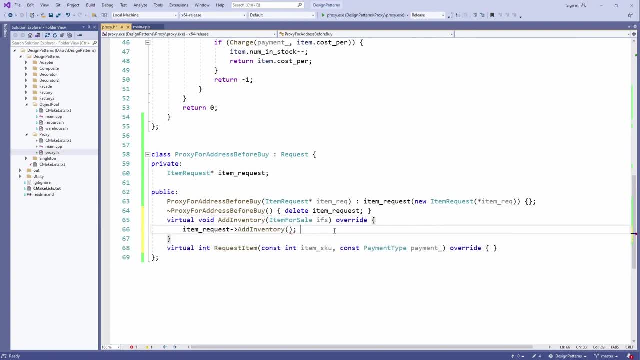 it to there. Does that make sense? That's this one And same thing here, But the whole point of the proxy is to do a little additional stuff. So that's probably what we want to do, and have some private functions. Let's do a check payment here Now. we said that this is for address. 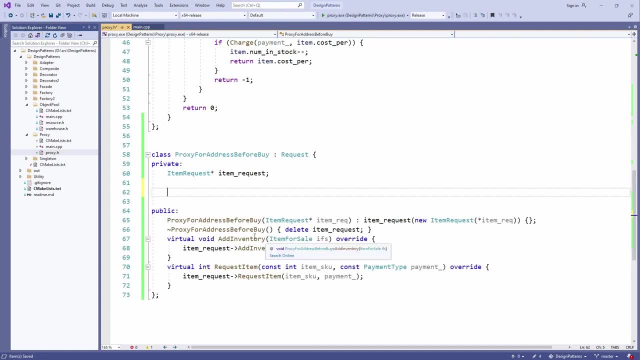 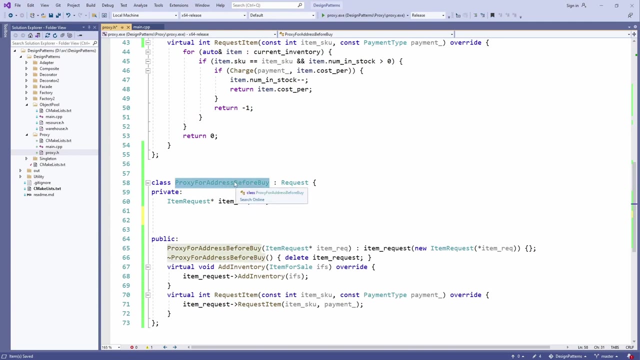 So you know, we could add on an address and write a whole new function for all of these that does such a thing. But let's keep it a little simpler. Okay, let's, let's just make this: check a few things Before doing the request. Check before item request: That's what we're going to call it. 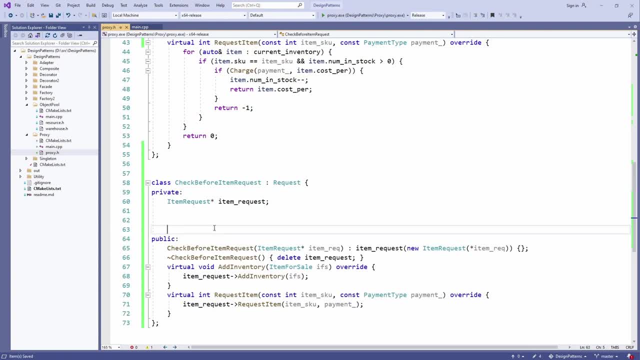 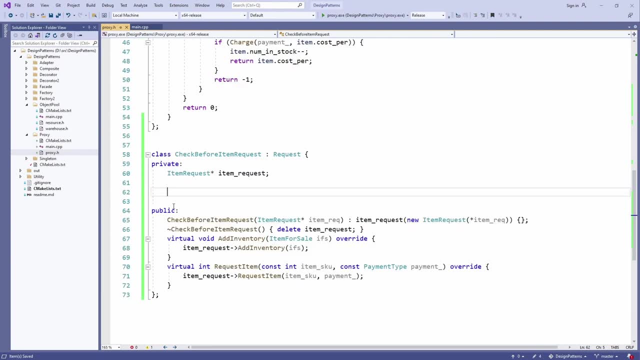 That's what this proxy is going to call. So forget about the address. we're going to totally skip over the address factor overall. of course you'd want to work that into your real system, But let's keep the complications down. So what we want to do here? if we add inventory, 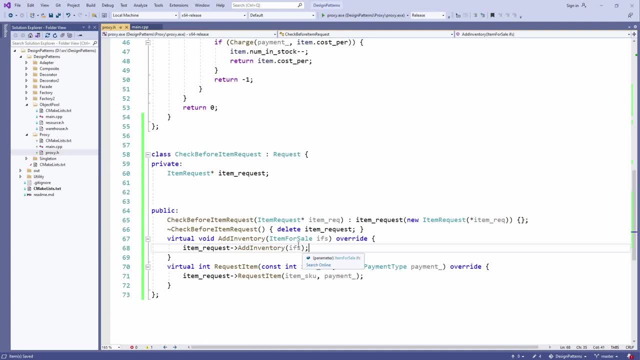 for example. that can probably stay the same. We could add a check before the item request, But let's keep the complications down. So before and after: if we want Yeah, let's actually do it. Let's say maybe we want a. 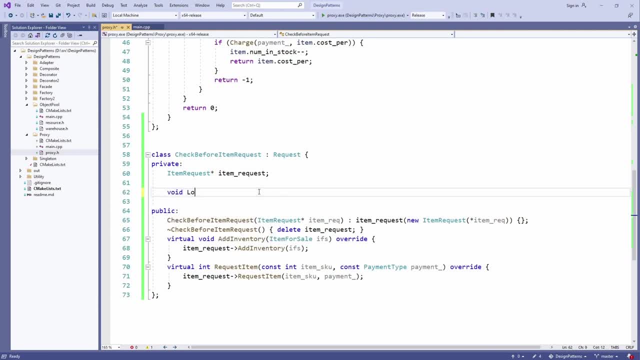 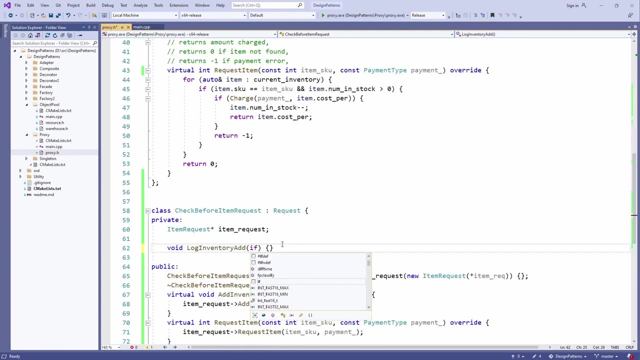 little bit of a log. So let's go void log inventory And this will just take in the whatever details about it. So, rather than being function, obviously we could even just put this code right here, because we're going to call this. 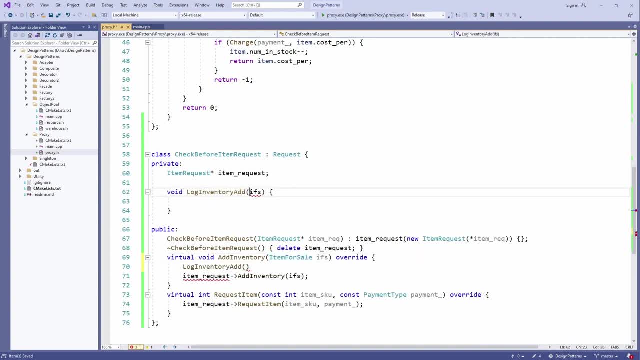 and we're just going to say we'll just do a CL and pick to add. you know we can, you know we can put further checks in here to say like if it added and all that kind of stuff, we can do a whole bunch of additional queries up in here. 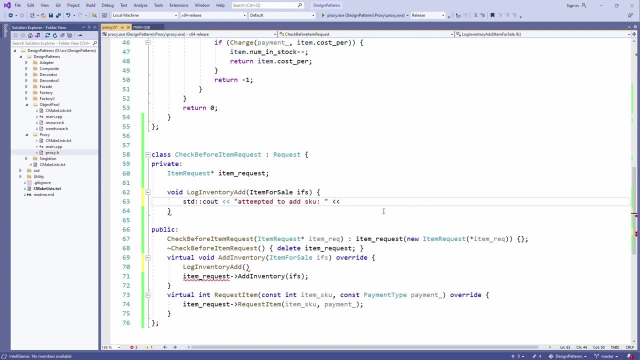 I'm just going to keep it simple, but we might do it before and after, see if it actually got added that sort of thing. but for sake of time I'm going to kind of skip over that and just put this: this quick attempted to add SKU, so 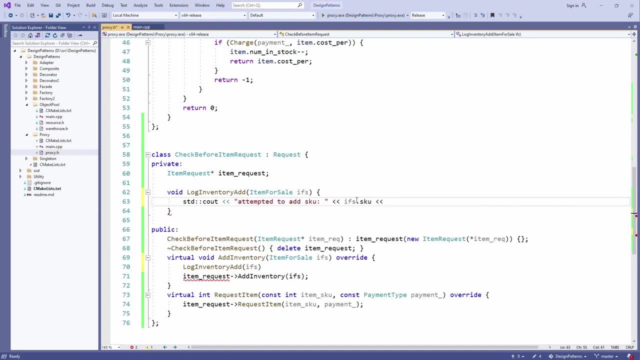 that should give you an idea, because essentially the rest of the stuff would be the same. so now we still have an add inventory, but now it also logs. so that's one thing you can do, and we can do the same thing with this request item, for example. we could have a 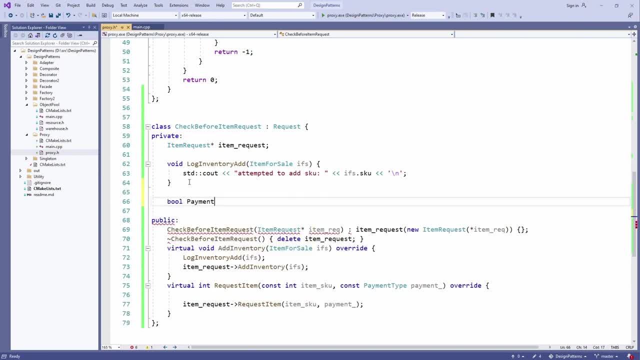 payment check or something in terms of true or false, just takes in this payment and we can do the same thing with this request item. and we can do the same thing with this request item and we could do our own pre-check on the payment if we want it, before trying to actually charge. 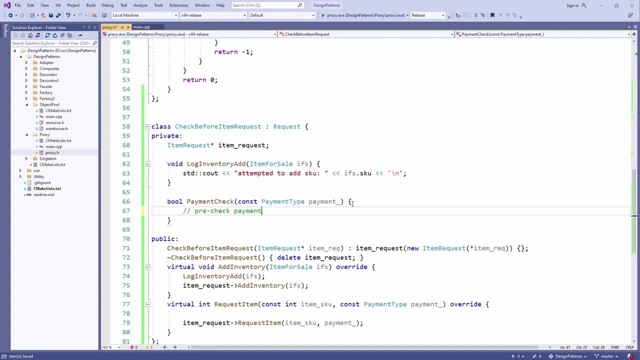 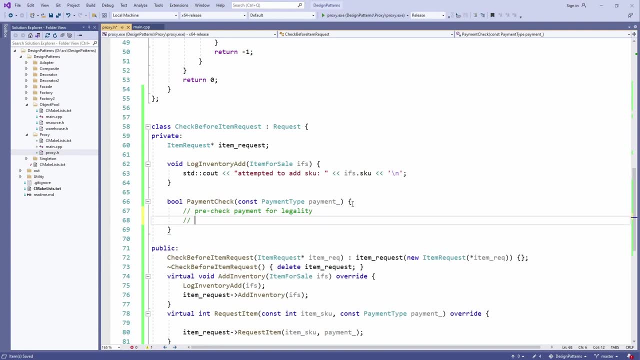 pre-check, payment for legality or something you know. just some basic stuff: make sure that the card isn't expired or something like that. make sure account exists, slash card isn't expired, etc. we're going to assume pass for now. so we're just going to return true for now. 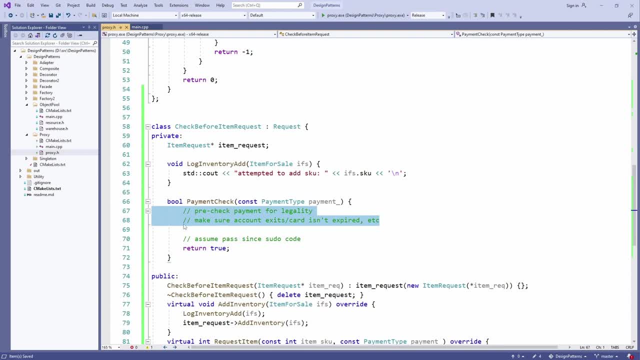 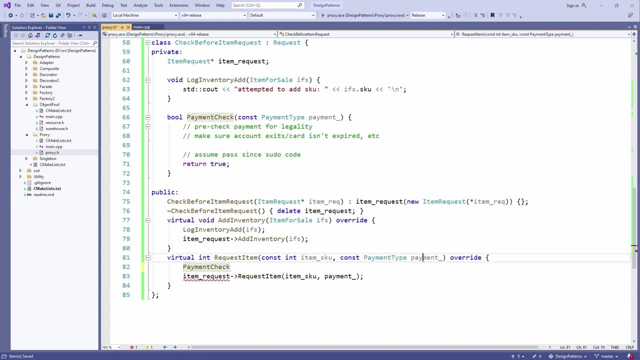 but pretend this was the elaborate system that did some additional checks, right. so we, you know we could do that here, and the reason this would be good is we could not even like- maybe we don't even want to send the request, like if we know that the payment is not good. 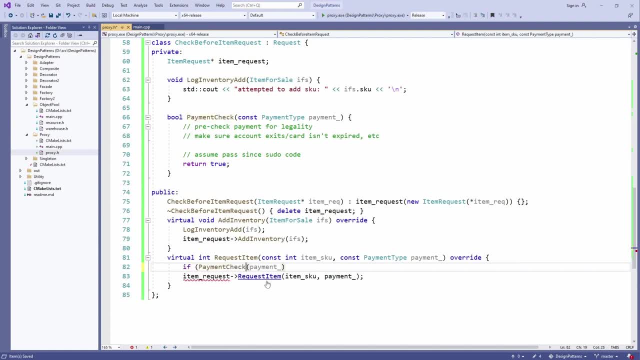 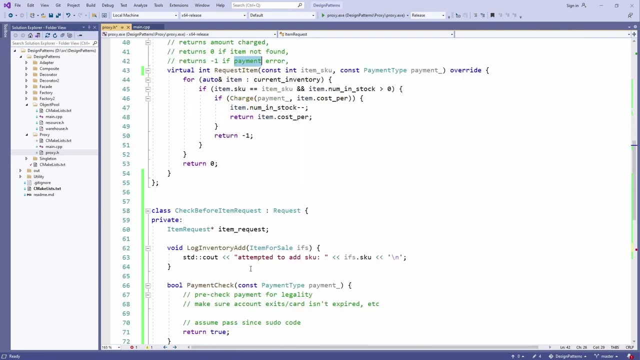 let's not even go further. so we could go if so, if not paid. so if this returns false, then we would return. I don't know we could go ahead and stick with the original payment error. we'll return negative one a little sooner. here it's a little proxy check. 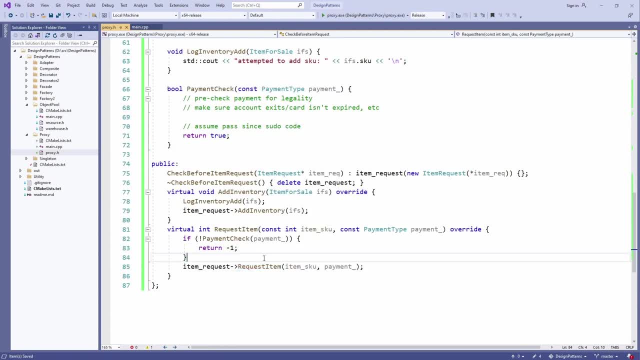 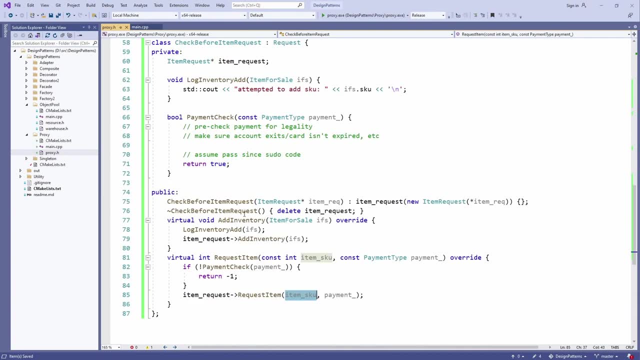 and we could also, if we want we could, we could do a initial query on the items queue. maybe- I don't know- that's going to be kind of hard because the way we got it worked up, but that's the point of this video. the proxy here is to basically be able to add some functionality. 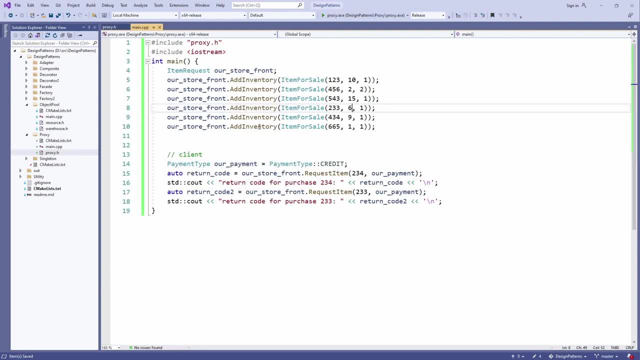 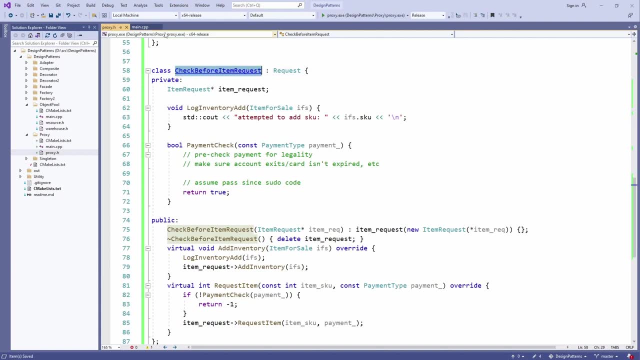 and pretend to be the interface that you want. so let's have a look back over here. so we have our storefront. it's got items. what if, instead of item request, it was now the check before item request? now you can see that it doesn't really like this right. 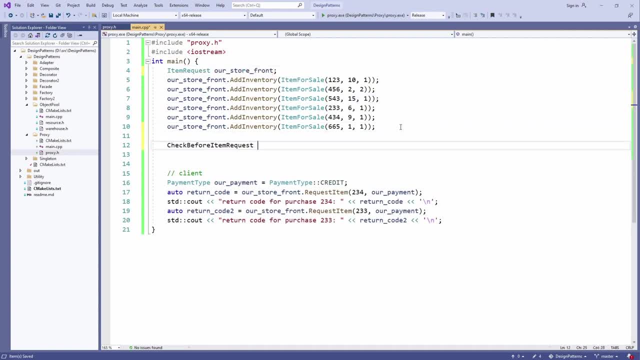 okay, so let's put the old one back. let's go now. let's make this proxy store now, of course it wants the same one, so or it needs, it needs something to instantiate and it wants a pointer, so we're going to have to do a reference here. 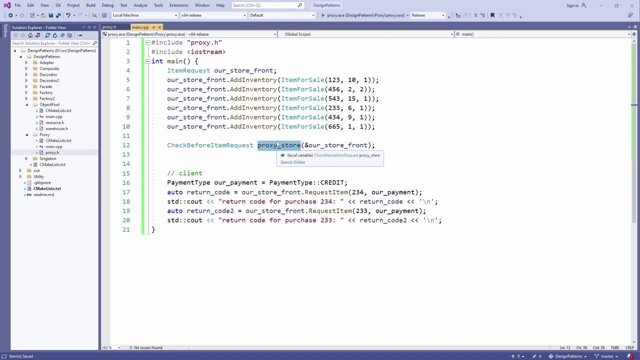 there. now we've got a proxy store and we can still do the same thing on this proxy store instead of our storefront and get some return codes and whatnot, so let's go ahead and have a check of that. we've also got new add inventory functions. 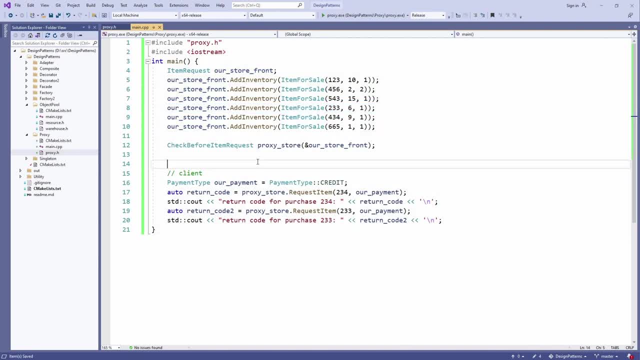 so we could test one of those. let's go ahead and just put one down here and this one should log. let's just add some different details: nine, uh, let's say two, in stock, so make sure to go: proxy store here, proxy it real store, proxy of it. 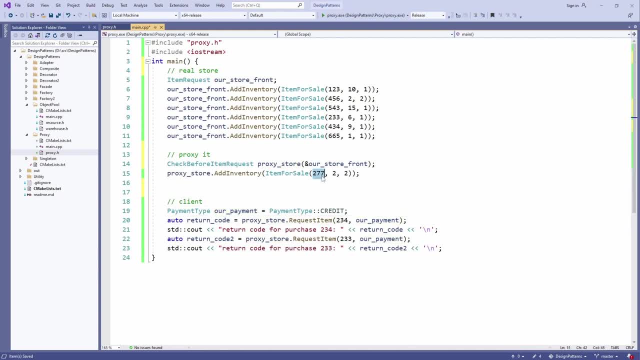 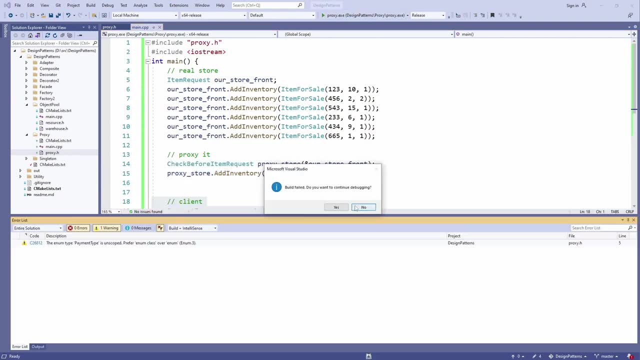 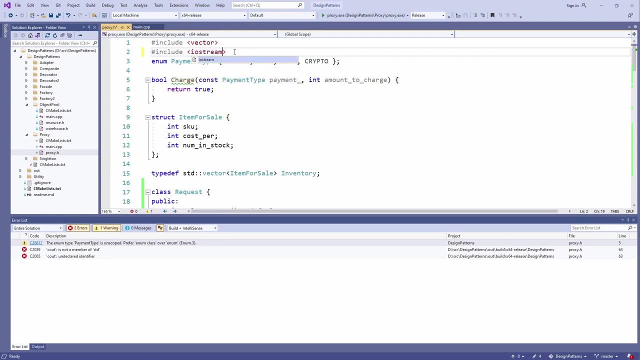 and here's our client run through the proxy. okay, so let's have a run of this code. we should definitely see the add inventory. these should work just fine and uh, well, we got an error. okay, so we need to include iostream in this header. i believe we have a c out somewhere. 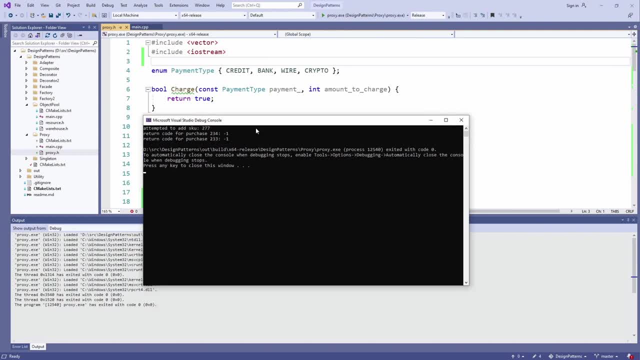 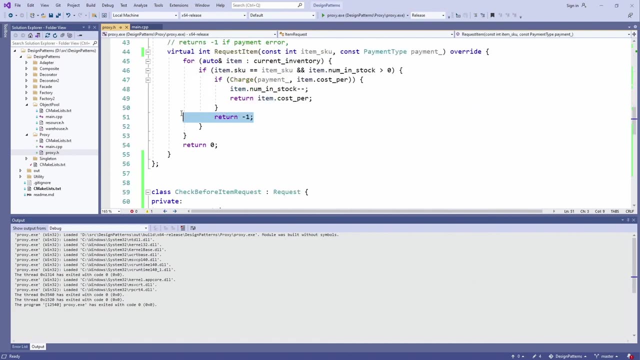 and i'll say play. and there we go. so we got an attempted to add skew. so that worked okay. we got a couple return codes, negative one. now, i didn't really expect this. i thought that one of the return codes would be successful. we're getting negative one. 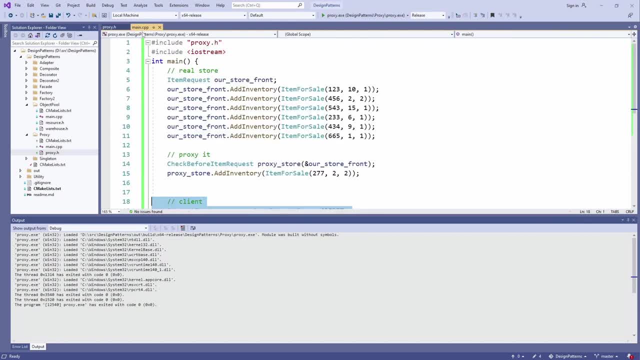 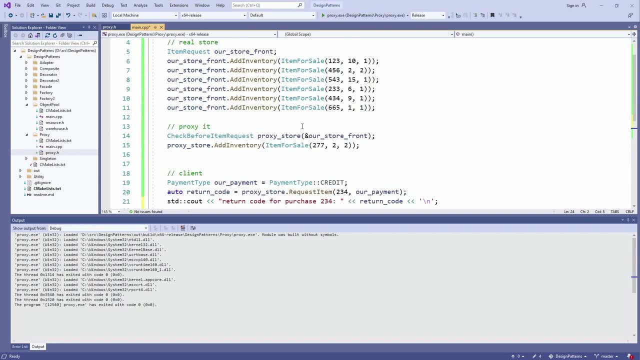 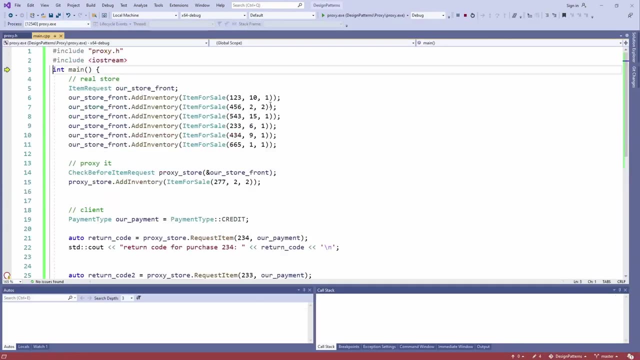 whereas item is not found. so there's something happening there that's not working quite right, because this one should work okay. so we can put a breakpoint here, put this in debug and see what's going on, hit f11 and then, uh, hit f5 to go all the way down here. 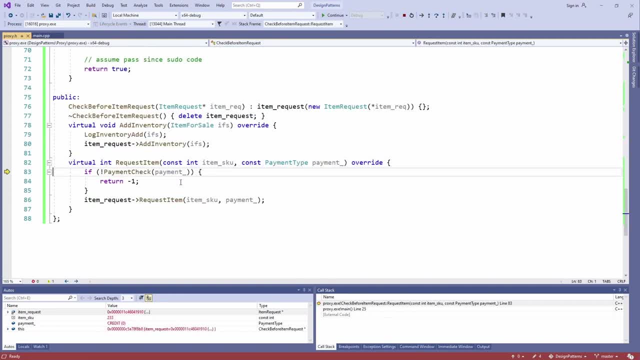 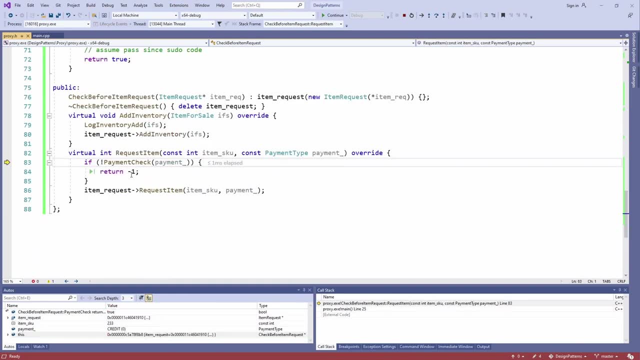 and then f11 go into this. let's see what's happening here. looks like our payment check is not, might be backwards. it's returning true, which turns into a false skips over. very good, uh oh, we're not returning here, so we should be returning that, because we want to return whatever this returns. 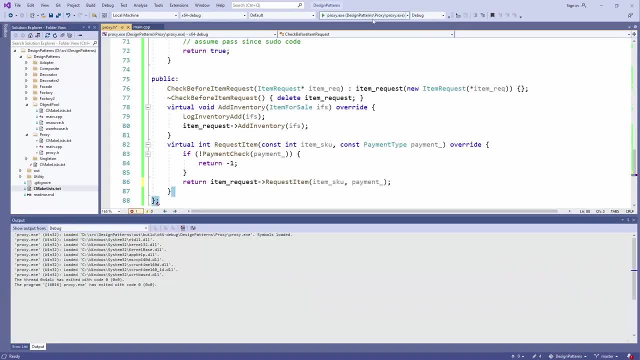 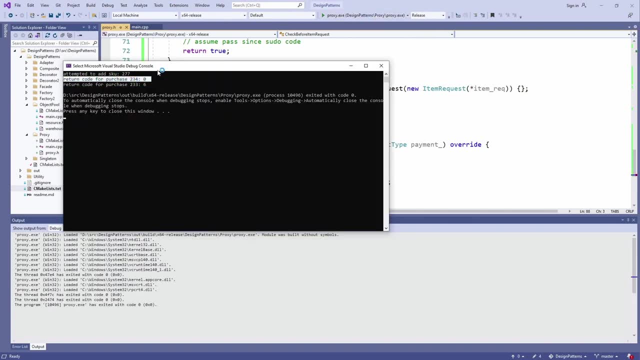 so that's the entire problem with the code. i believe it's a stop. go back to release and hit play. now it looks better, more like what we expect: turn code zero for the one that's not found, return code six for charge six and uh, that's doing it through the proxy. 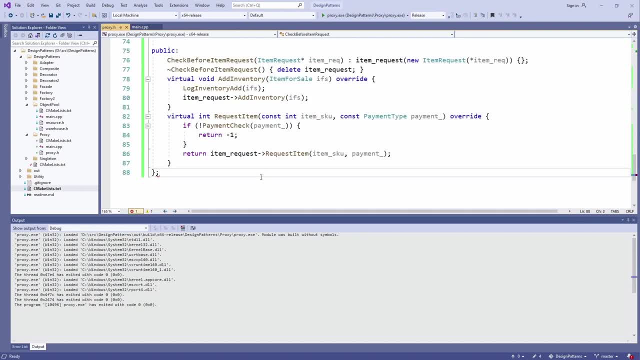 so you can see how proxies could be interesting and also scary. for example, a hacker might put a proxy over something and just skim a little of the payment off the top, or something like that. but uh, you know, that's the scary black hat of the whole operation. 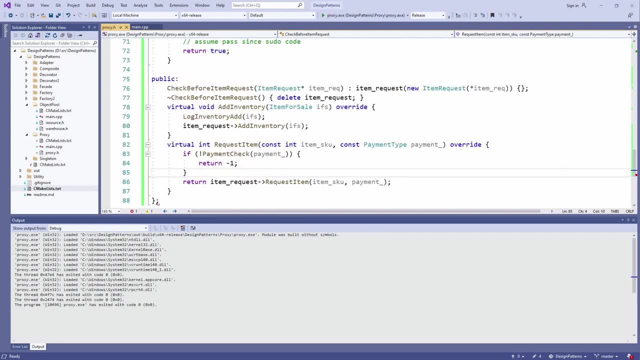 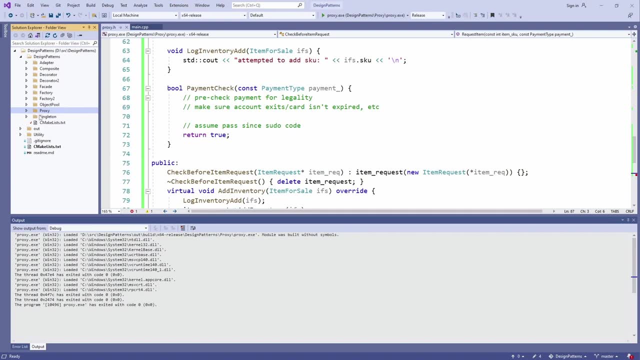 but generally you're just adding some functionality. i hope you guys have enjoyed this episode and have a better understanding of what a proxy is and how to implement it. c plus plus. this code will be up on github. if you enjoyed the video or learned something, consider hitting the like button.